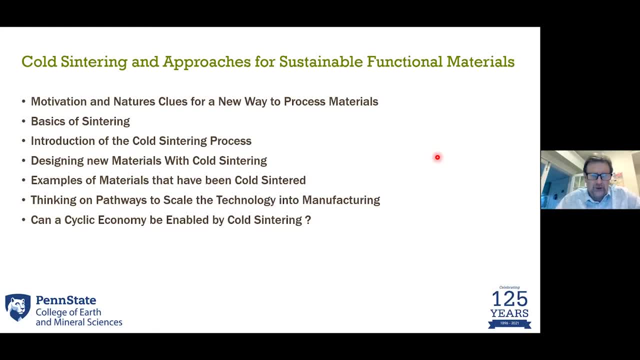 I will introduce to you what the cold sintering process is, how we can design new materials with cold sintering and give a number of examples of devices and various different materials that have been now fabricated with cold sintering over the last six years or so. 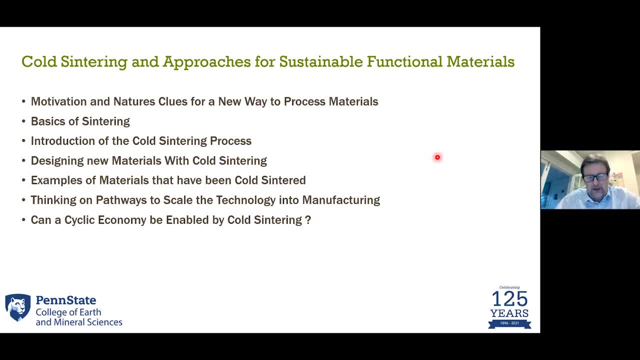 And it offers new pathways to think about how to scale the technology, And I'll show you some of the preliminary results that we have as we step down the translational part of taking stuff from the laboratory into the next stages for prototyping, And then, finally, there's a lot of discussion. 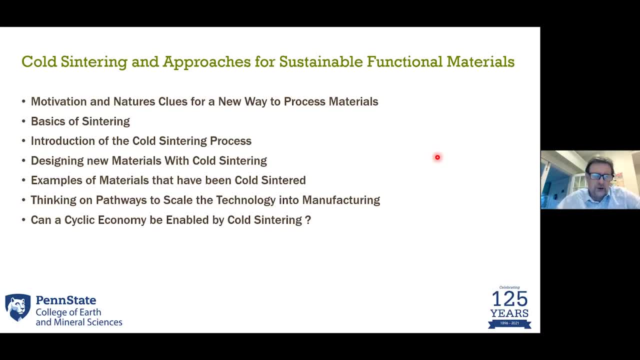 on resources, critical resources and so forth, And I'll point out- or I should rather accurately say, a colleague of mine, Dr Enrique Gomez, has pointed out- that cold centering can sit at the center of a cyclic economy, And I will talk a little bit about those ideas as well. 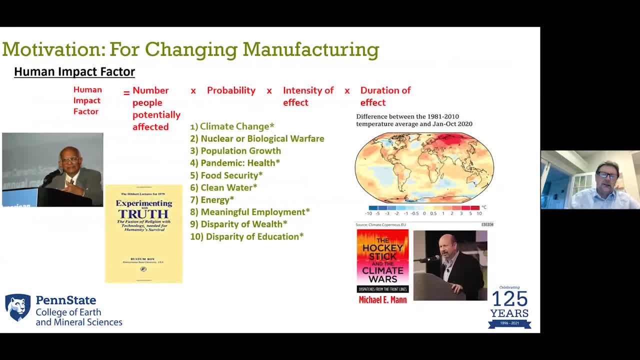 that we are working on So motivation. So, as I said, I've worked on electro ceramics for a long time And certainly I've worked on electro ceramics for a long time And certainly electro ceramics have implications for battery capacitors, fuel cells. 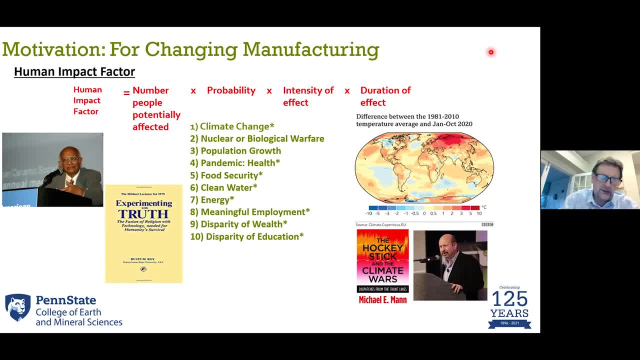 and many other forms of materials and devices that potentially can help the overall climate issue. But at the end of the day, it is very important for every scientist- young scientist or old scientist- to think about the reasons for doing research, but thinking about humanity and technology and the importance of not getting lost in your graphs. 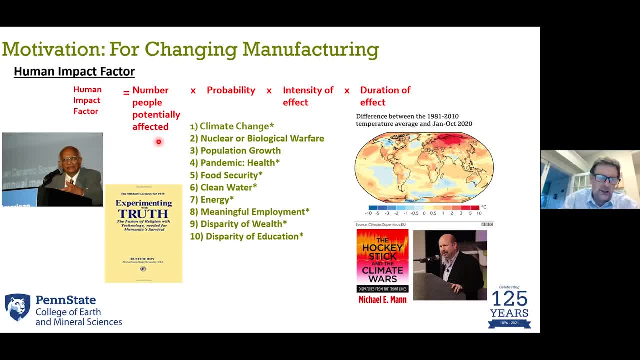 and in your equations. and certainly a old EMS student at the time in the 1950s, Rustem Roy in geosciences, who then spent his whole career at Penn State really driving interdisciplinary research, really got us over those years to embrace complex problems and I pulled upon one of his. 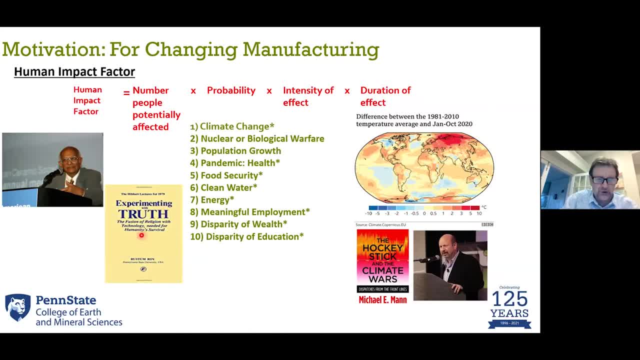 books. one of his many books, this one's called experimenting with the truth, the fusion of religion with technology needed for human, for humanity's survival, and this is a rather intriguing book, written in 1976, and one of the things contained within it is this rather interesting. 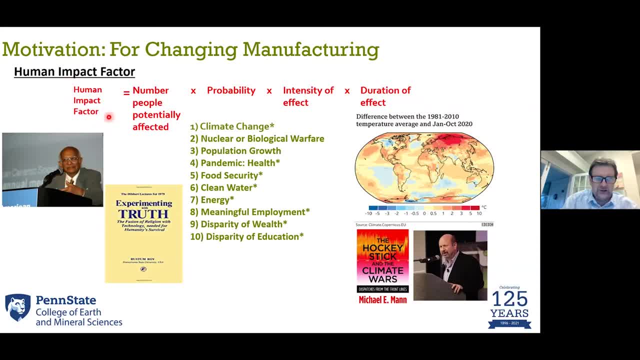 human impact factor equation, which has whatever the impact is, is being influenced by the potential number of people being affected by a phenomena, the probability of that event, the intensity of that effect and the duration of that effect. and back in the 1960s he sort of almost had the same list as this. it's been. 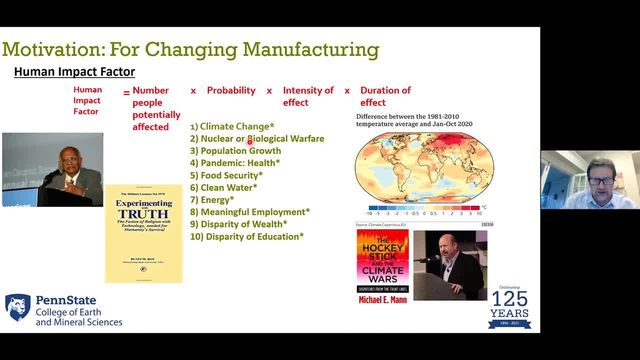 updated with some insights that I've put to it. but at the top of his list was nuclear biological warfare, which is given in 1976. you know the height of the cold war. this is probably not a surprise, but I would argue that that now some of these issues are there. probably the top issue is climate. 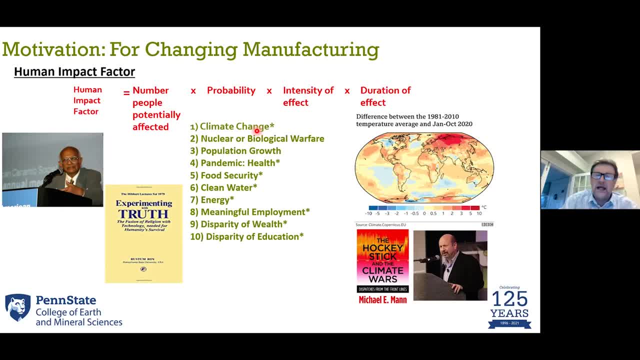 change. so, as a material scientist, how do we now help to address climate change? there's really got to be through our production and also through our engineering. I will point out that one of the biggest sources for for co2 emissions previously was lighting, and since the development of solid-state lighting, that is almost off the top 100 list in terms of drawdown. 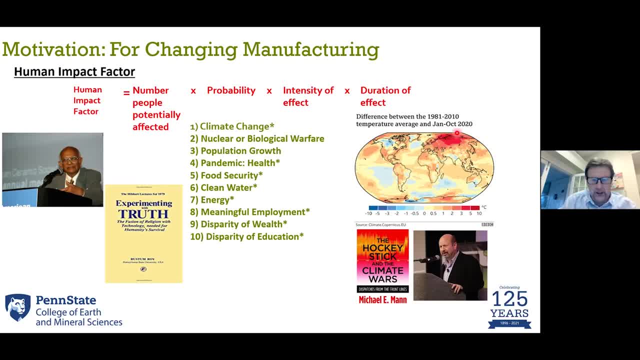 strategies, also being in our college. you know, obviously we've got fantastic climate scientists. everybody knows that there's a very, very strong group in here- one of them is Michael Mann and certainly people like myself- that follows data and follows data. from this group you can see the significance of the hockey stick, data translation and looking at the anomalous 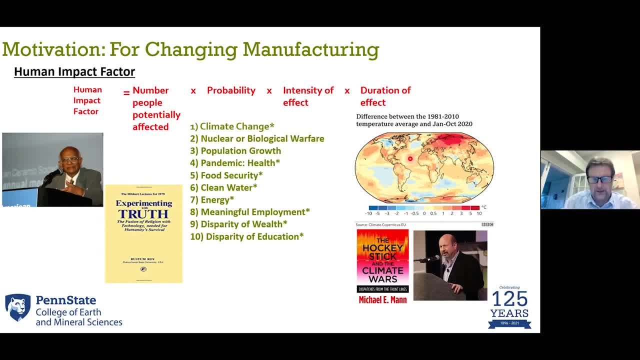 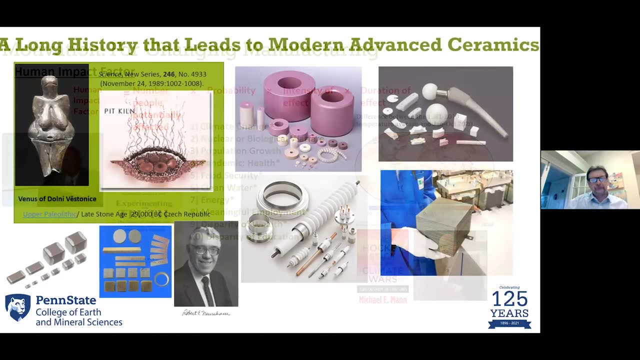 climb of that type of data is absolutely petrifying to people that are data driven, and so one has to ask: what can I do for our future generations? and it's that sort of motivation that got me thinking differently about how to process materials now, the sorts of materials that we're talking about. 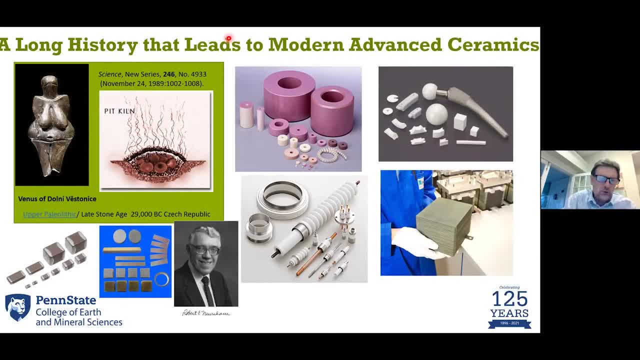 here is ceramics, and ceramics are actually the oldest of the of humankind manufacturing, from at least an additive perspective. I don't know if you've ever seen this lady here before, but this was found in the Czech Republic and has been carbon dated to be 29,000 years BC, so mankind. 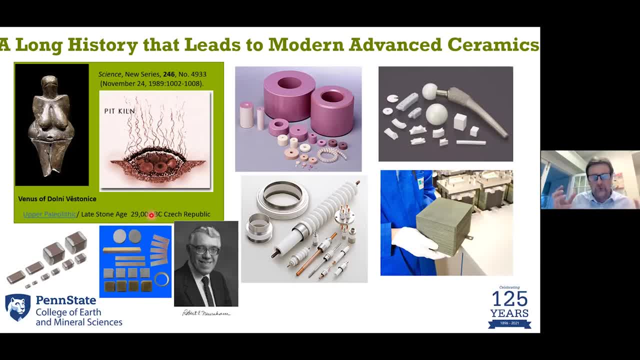 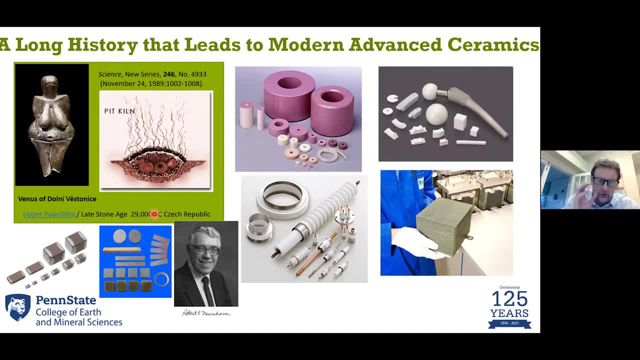 really hard to contemplate in terms of the age of materials, but that was probably the first synthetic process that um, that stone age man basically did in um, in it, um, in such a long time ago, and obviously there's many examples that translate many, many of the materials that we've. 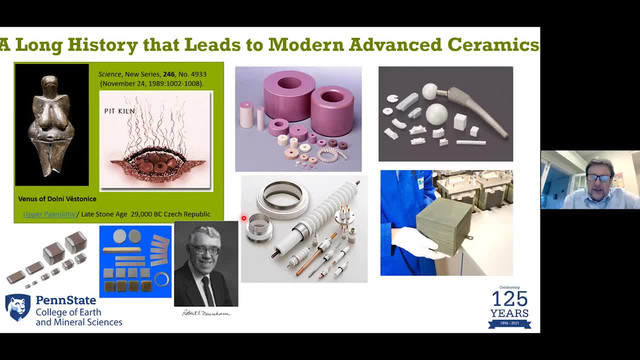 been using in the last 50 years, and so we've got materials like this that are used in microwave technology, um, bioceramic materials for hip implants, insulative type materials, capacitors. over four trillion of these are made out of ceramic material. there's probably a thousand. 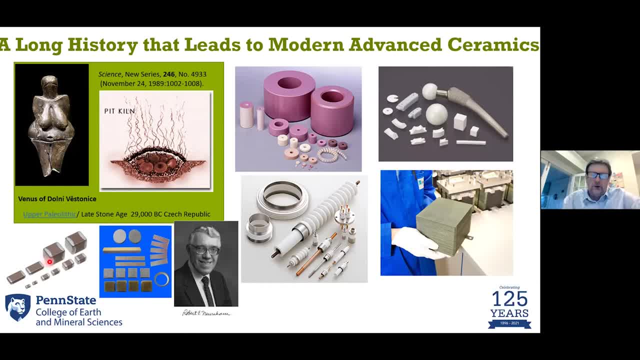 of them in your cell phone, and these are the sort of areas that I work on. this gentleman here was an inspiration to many of us in our college and in our department. it's Bob Dunham. he was a national academy member and he developed piezo composite materials that then basically, if 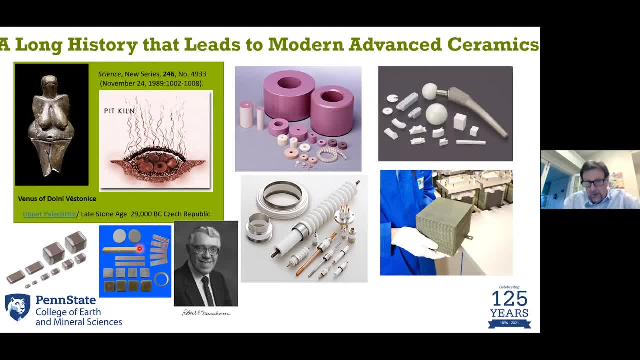 any of you have ever had an ultrasound. it's that technology that he won the Franklin medal for. that is there and it's again an electroceramic and any more energy related applications. there are things like fuel cells and batteries that are now emerging within this field. 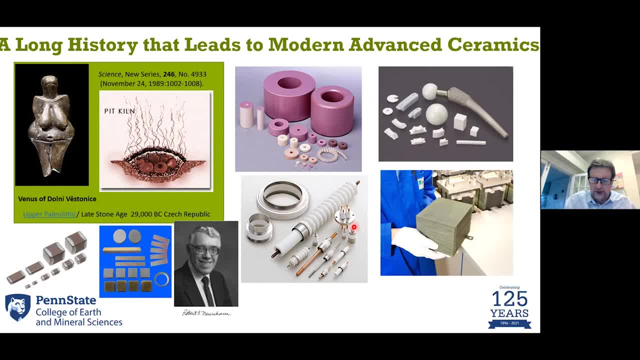 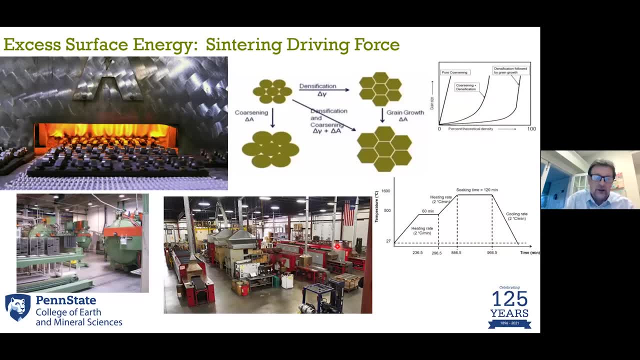 but all of these materials are all sintered at very high temperatures. I use furnaces in a factory floor like these different examples here all over and and and. they generate enormous amounts of waste, waste heat in the densification process of these ceramics. remember taking these powders and then driving them into a dense monolithic sample going. 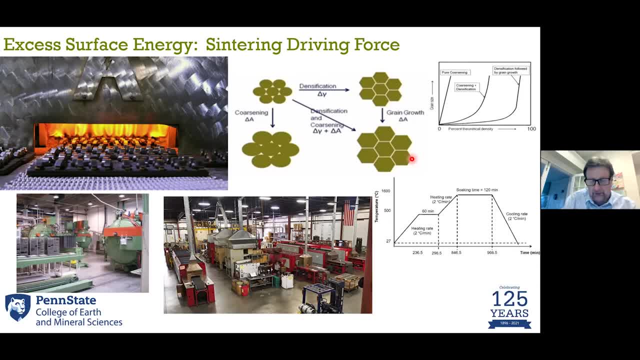 from about 40 percent dense to about 98 percent dense and then driving them into a dense monolithic sample, going from about 40 percent dense to about 98 percent dense and in doing so being driven by the thermodynamic process of minimizing surface area and the sort of temperature profiles that 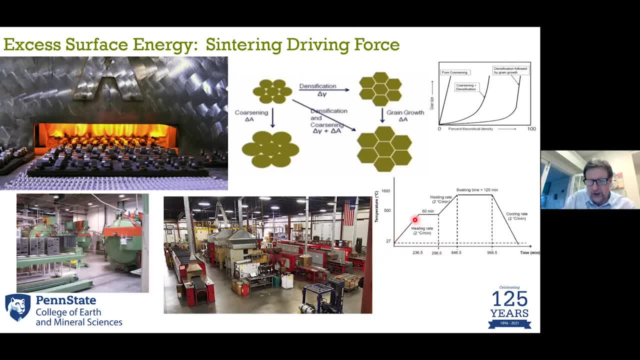 these furnaces take is processes that then remove organics, say at 500 degrees, and then driving a temperature up to temperatures such as a thousand to sixteen hundred degrees celsius. just imagine the heat that is generated from your oven when you're cooking a pizza at 450 celsius. this is so. 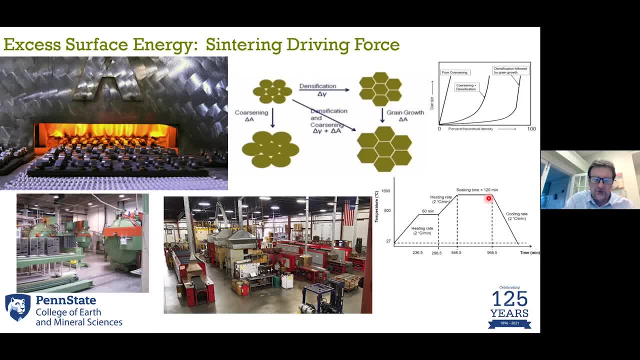 450 fahrenheit, not not 1600 celsius. so enormous amounts of heat, enormous amounts of heat loss, enormous levels of inefficiency, and if you are paying the bills for these processes as a manufacturer and an engineer, you are also basically costing your company a lot of money. 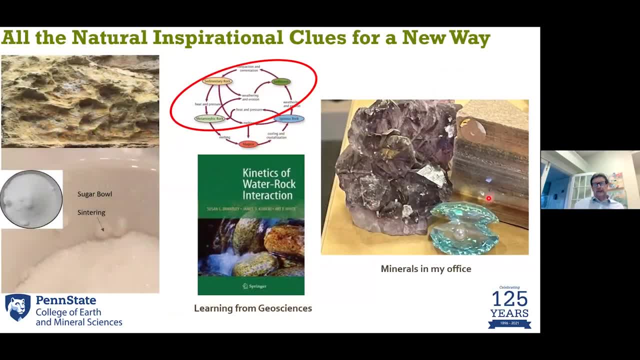 in the fabrication of such a process. so is there a different way? and this was a question that i asked myself over eight years ago, and there was a lot of reading that i did, including readings inspired by some of our colleagues, like sue brantley and others i had 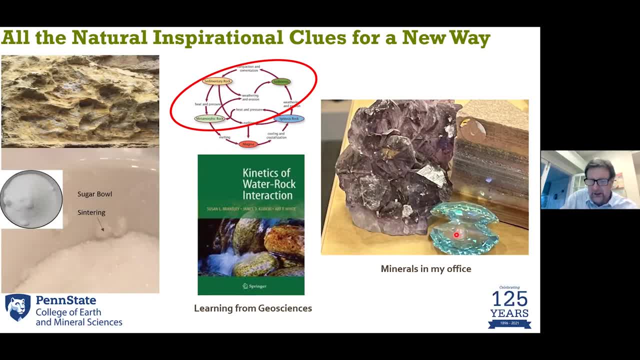 minerals in my room. you can see here some quartz. i had a pearl, which is a biomineralization process, and some sedimentous rock that i got from dresden on a trip once and there are many, many clues that how these are made are not made in a way naturally. 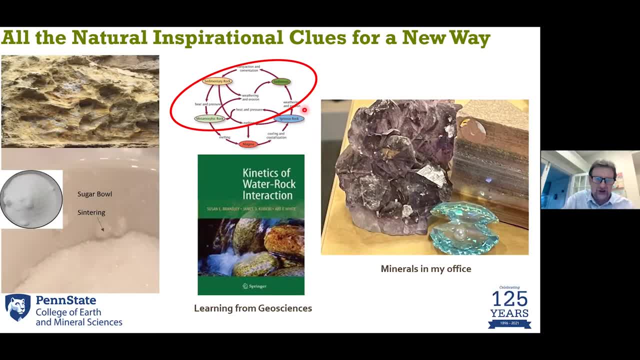 they are made in a way that uses a furnace. they use processes such as weathering, pressure and solution, precipitation and methods like this to then drive it, even sitting in a damp kitchen in in, say, scarborough in england at some time. looking at a a sugar bowl, you can see that the crystals 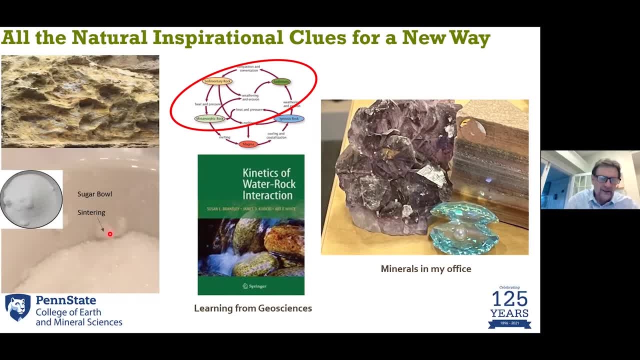 are undergoing a densification and sintering. all these are clues that the people who are working in the industry are going to be able to find. all these are clues that the people who are working in the industry are going to be able to find. there may be a better way to center materials. 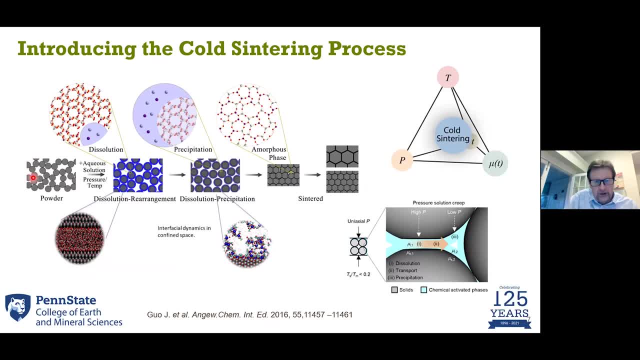 so the basic process is the following: there is powder, we add a liquid transient phase, we apply a pressure, we add a moderate temperature and as that liquid touches the surfaces of these powders, it drives a dissolution process, the same way as sugar is. is is dissolved into your 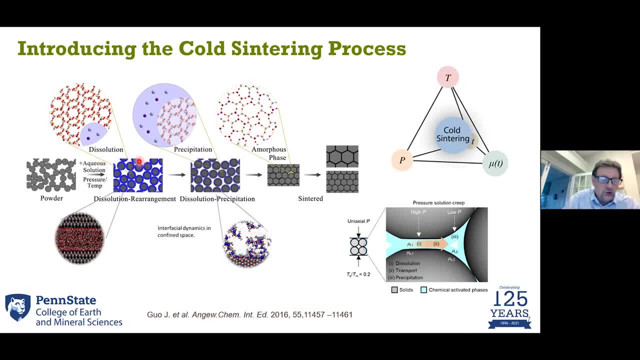 into your warm cup of tea this evening, um, and then, as you then evaporate that off by by a heat treatment, driving it towards the evaporation of water, say a thousand, a hundred degrees, then that sugar then super saturates and then re-precipitates. in this case, you're driving. 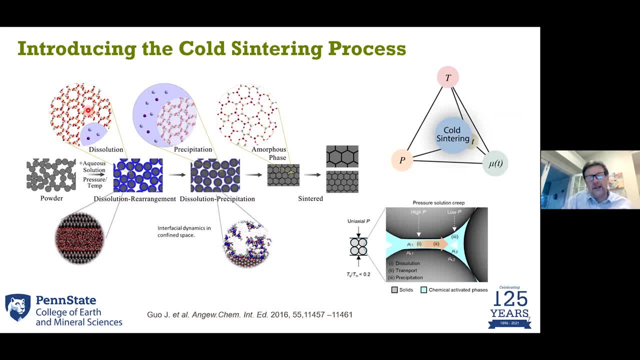 the surface into a solution in the liquid and then you're basically super saturating it and it's re-precipitating and the dynamics and transport of all those processes then allows this to then densify at temperatures previously unrealized, like 150 degrees celsius at um. 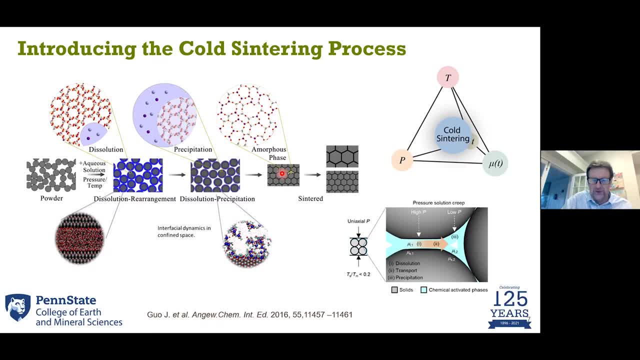 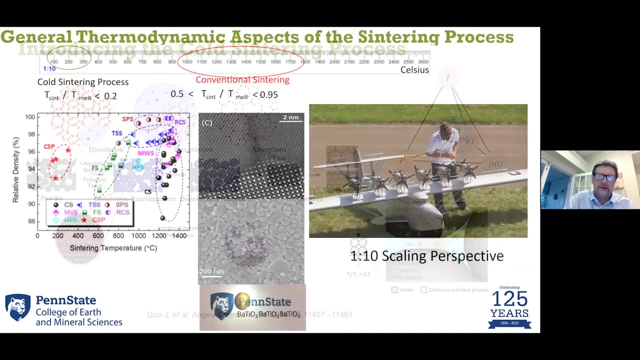 and in also very short times. and so these dynamics of really low temperatures, applied pressures, moderate pressures, anywhere between 70 megapascals to 500 megapascals, not geopascal levels, the activity, the all-important chemical activity, in time is critical to this densification process. so if we consider like a scale here, uh, in terms 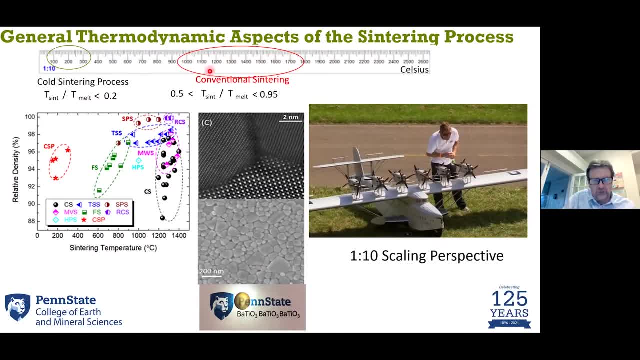 of celsius. most sintering of oxides are in this range: a thousand to seventeen hundred. the cold sintering allows us to work right down here, so it's like a ten to one ratio. in fact, the rule of thumb in a textbook is the sintering temperature. over the melting temperature lies. 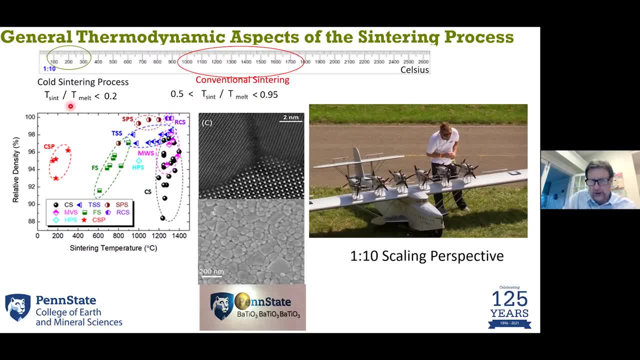 between 0.5 to 0.95. cold sintering is below 0.2, often 0.1. so in the case of barium titanate this is called cinder barium titanate. you can see here beautiful triple points between three adjacent grains. 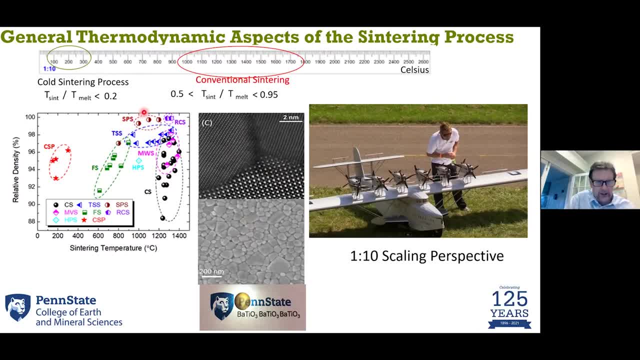 dense microstructure and um. and then here is all the best in class of all the other fancy techniques to sinter, including spark, plasma sintering, microwave sintering, conventional sintering, etc. cold sintering is over here: much lower temperatures and also significantly faster times. so we're 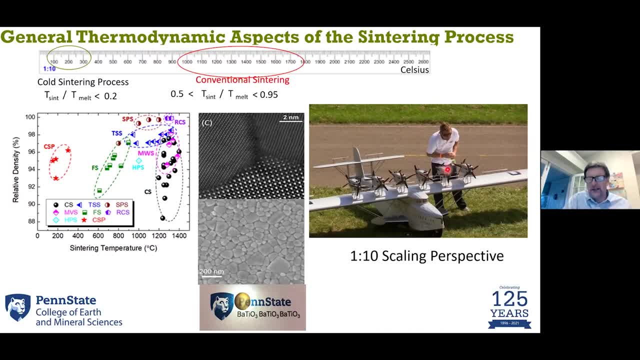 looking at 10 to 1 change in the total energy, if not greater, at least 10 to 1. in terms of that, to give you one perspective in physical scale, it would be like this gentleman here looking at this aeroplane being reduced by 10 to 1.. so it really gives you a perspective. this is a massive 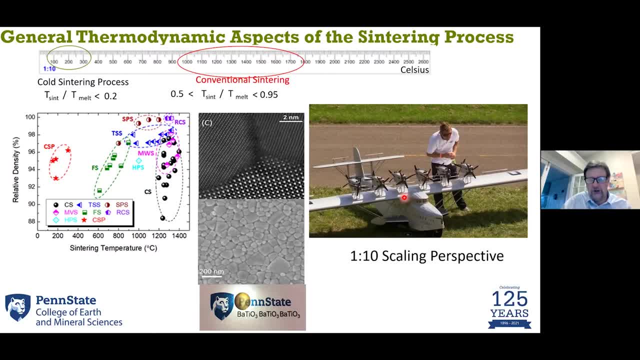 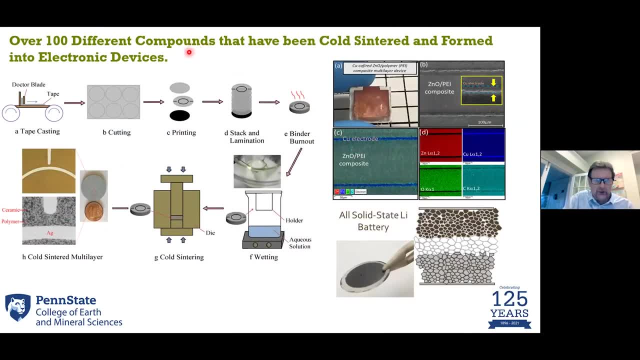 change that we have as an option to how to process materials and densify them. um, we've done over 100 different compounds now, not just oxides, but but a variety of different materials, and more than just densifying them as a ceramic, we've designed them in ways that we've. 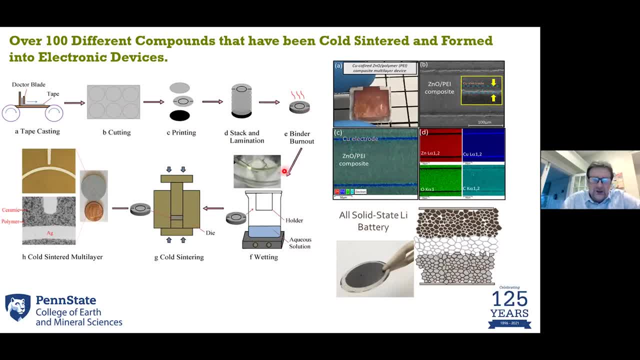 been able to do over the last few years. we've designed them in ways that we've been able to do over the last few years. we've designed them in ways that we've been able to do over the last few years, and we've also designed them in ways that we've been able to do over the last few years. 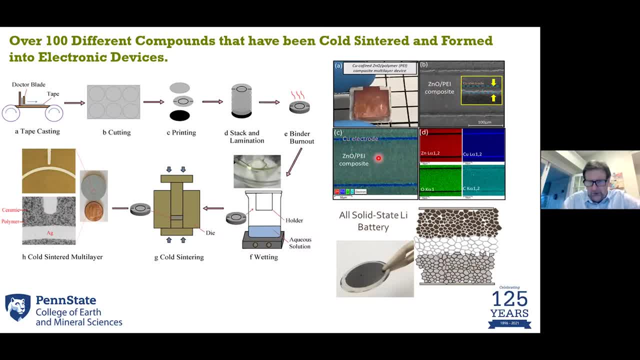 and over here you can see multi-layered type devices for barista being made, where we're also not just co-sintering the ceramic but also the metal electrodes, all within this same process, and i think this work was done at 150, and we're also 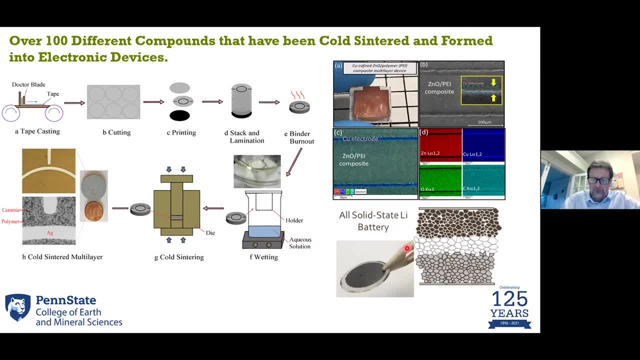 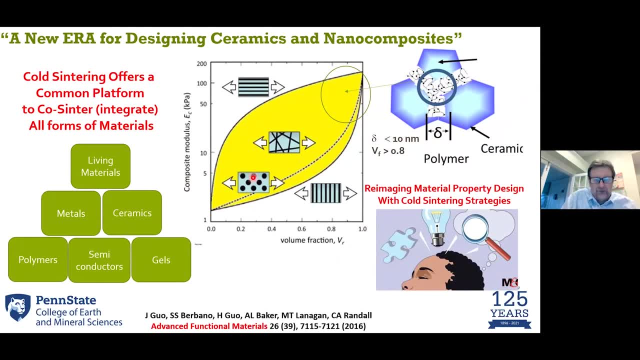 looking at how to assemble new solid state batteries with this same type of technology. more than just ceramics, what this offers. with this, basically severe reduction of the processing temperature of a ceramic, we now can push the ceramic processing temperature in the domain of where we do polymers, polymer polymerizations, cross-linking and flow processes with polymers. 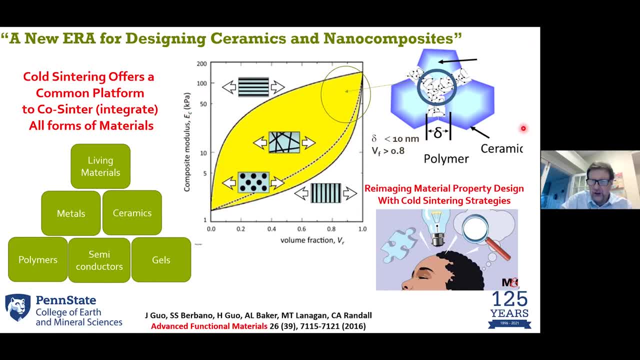 so now you can actually make new types of composites where you can put small amounts of polymer in the grain boundaries of the process- ceramic materials- to develop completely new nano composites with new types of properties. you can combine metals, you can combine semiconductors, gels, as we have in some of the 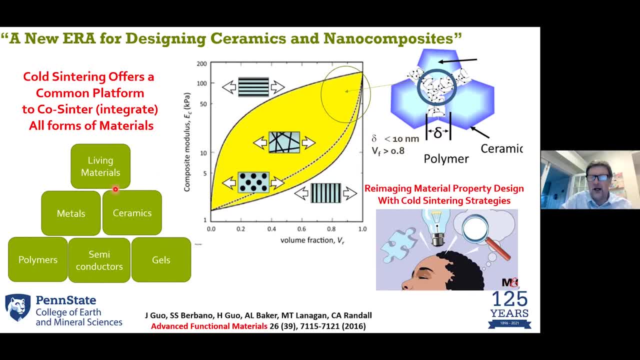 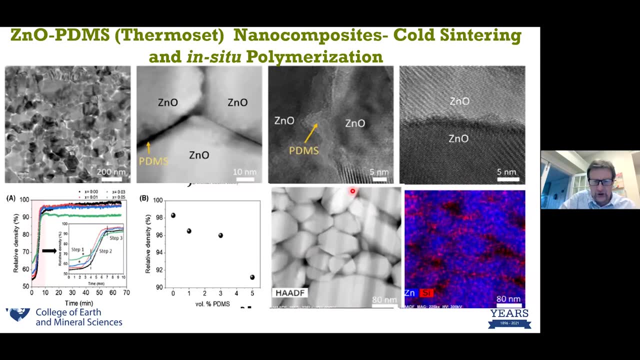 in some of the battery materials and in fact we're even- i have a colleague in england- even looking to incorporate living materials into the ceramic matrix at lower temperatures. so just to prove to you that these must be low temperatures. you can see here the densified microstructure, the sort of 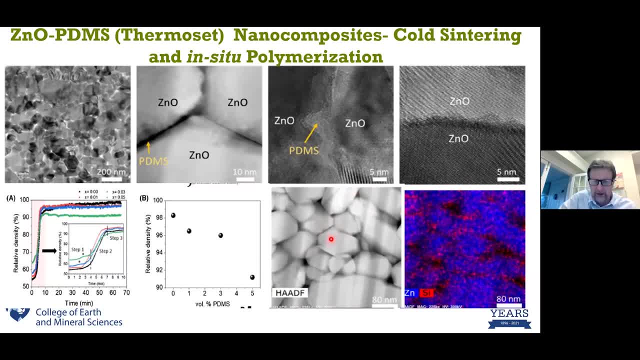 classic 120 degree angles between densified ceramics. but when you look more closely in the tm, in this particular case, there's a polymer around each grain, in this case a silicone- elastic only up to about five volume percent in this particular case, but still maintaining densities above 96. 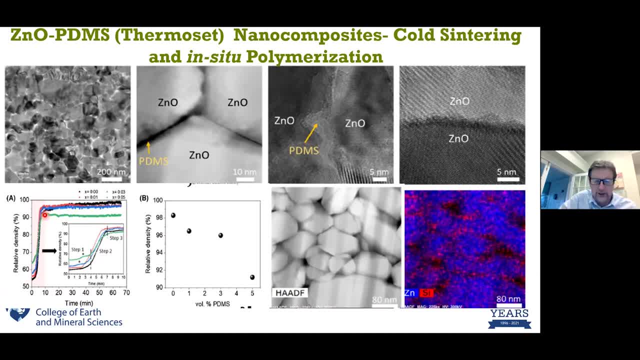 and you can see from the densification that this all happens within 10 minutes, right. typically just centering zinc oxide takes multiple hours, right, this is happening within 10 minutes and densifying the materials, but leaving a polymer also in the grain boundary, so you can have it free of polymer or with various different volume. 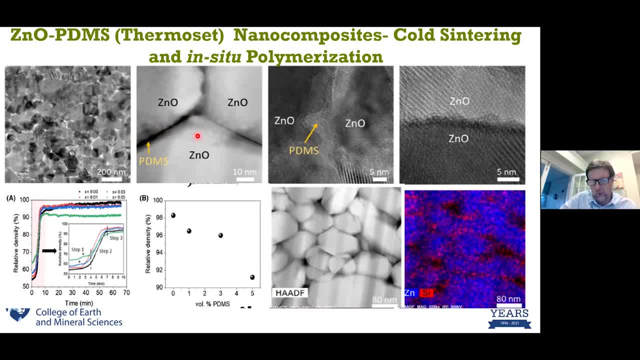 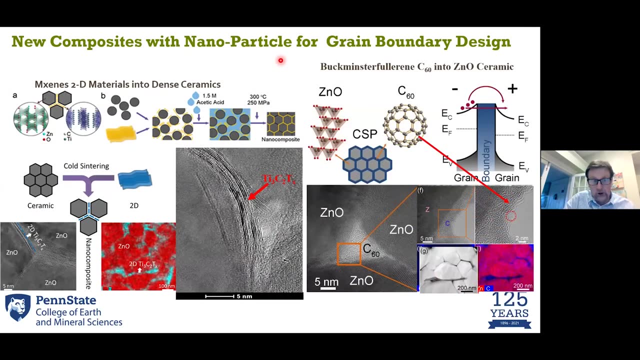 fractions of polymer and different chemistries of polymer all making up these types of composites. so it opens up the enormous way of which various different aspects of material science can interact within this processing platform. not just polymers, it can also be nanomaterials here. 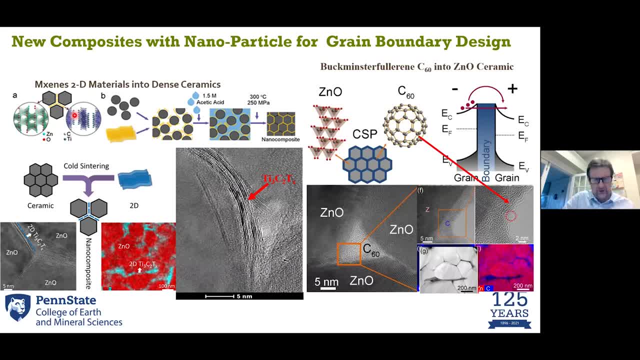 you can see some nano, so-called 2d materials. penn state is very, very big in 2d material. we've got over 50 faculty working in nanomaterials uh with with these 2d type type morphologies. so here you can actually disperse around your ceramic nanomaterials that are 2d in shape around each of. 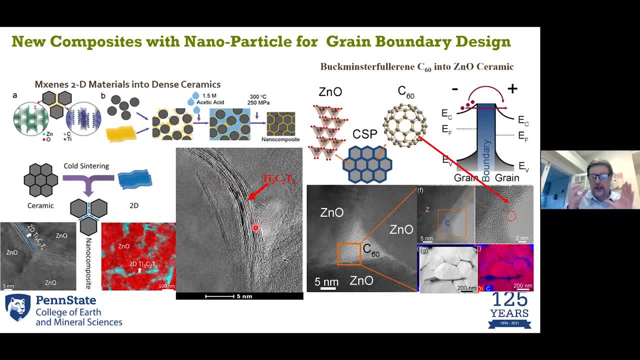 the individual grains and then center this whole thing together and trapping that in all of this sort of five nanometer scale. over here we've done the equivalent with the old-fashioned buckyball. okay, very, very similar. you see the buckyballs and the grain boundaries. 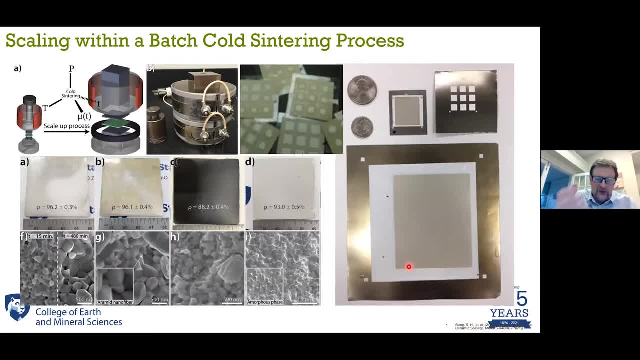 so clearly you can do a lots of different types of innovative things with these, but at the end of the day, if we are going to impact society, we've got to be able to translate it out of the laboratories, and so to do that, we're starting to look on how to print and 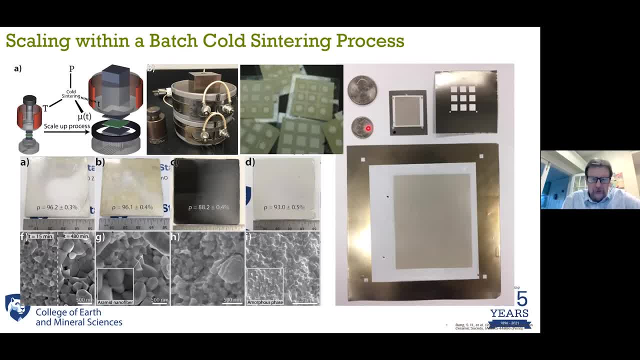 densify materials on different types of substrates- metals, plastics, how to make tiles on larger and larger scales but still having high densities. and we've started to do this now. even with thinking about a continuous process, which i don't have time to go into at the moment, it's still very much. 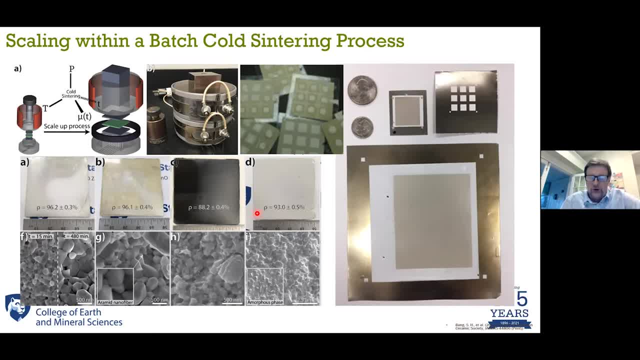 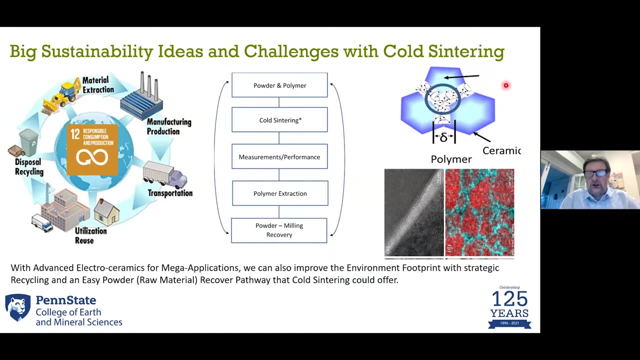 in its early days. but you can see there is a route towards the manufacturing of such a technology, to then be able to make new types of devices and to be able to scale them to impact society. and, as i mentioned earlier on one of my colleagues, enrique gomez, 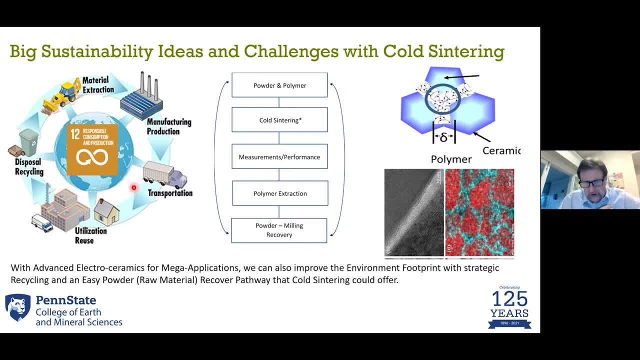 pointed out to me that this may be the ideal process for really creating a cyclic economy, particularly the fact that you can put polymers into the grain boundaries of a ceramic material, so you can make a material which is maybe 95 ceramic- two to five percent of. 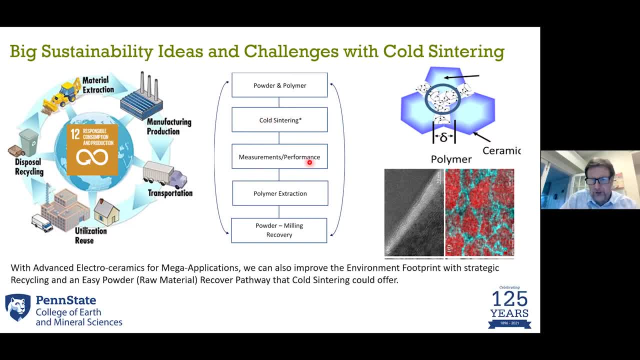 of a polymer. you can cold center it, you can have the properties that you almost almost would see with the normal ceramic, but then you can then do an extraction process to then get rid of that polymer, either by heat or by a solvent as extraction, and then recover. 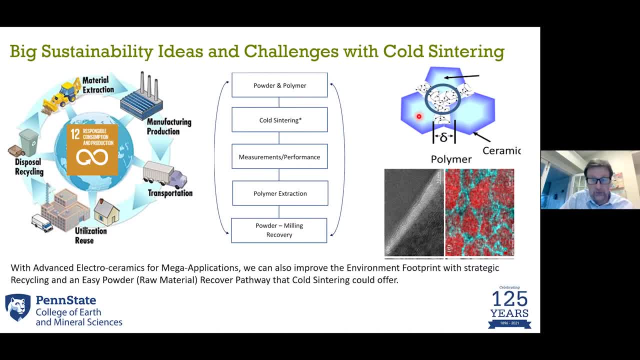 really the all-important materials that may actually have compositions with very rare rare earths. they may have, you know, very expensive levels of purity to those powders and you can take those, build them down again and then re-drive this into them. a reuse cycle, because again, after some milling, you could add it with the polymer drive, the cold. 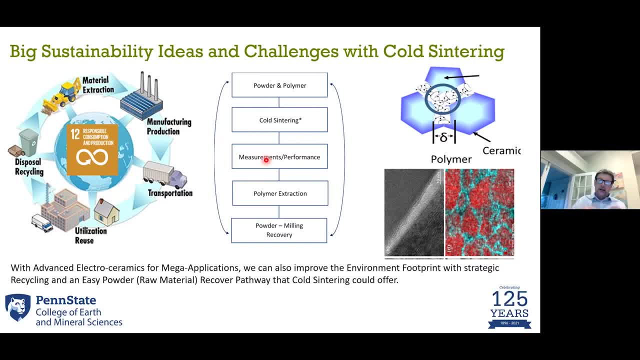 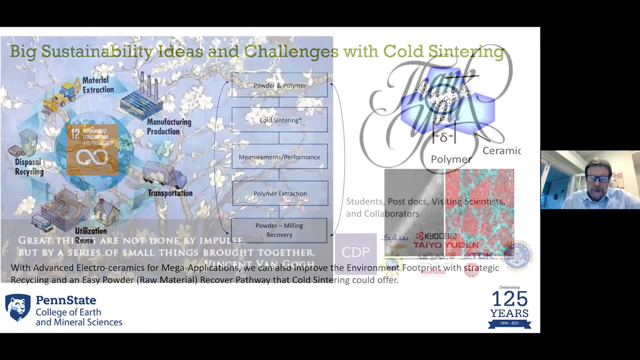 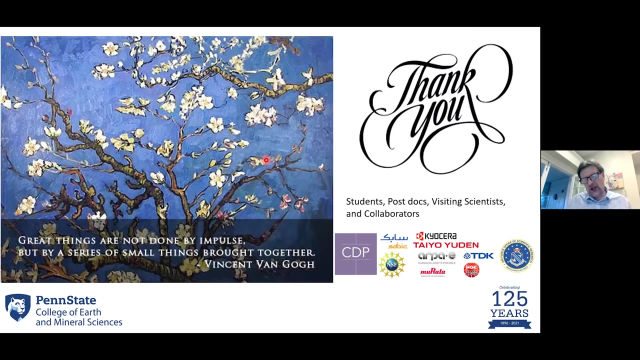 centering, make your devices again, and we're starting to do some of these types of demonstrations with some of the mega applications that obviously are there with electro ceramics, such as some of the batteries. okay, so, as we wrap up here this evening and open it up for questions, this is an idea that came to us. 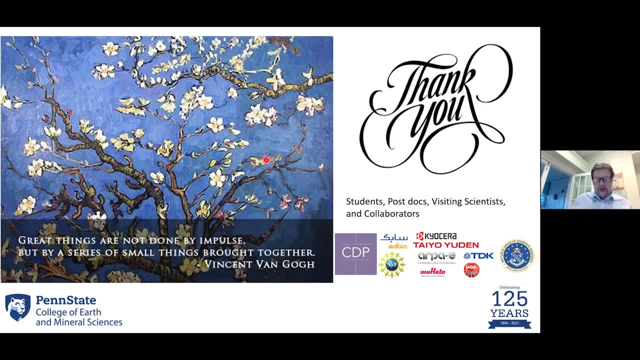 over six years ago- actually, it's more like eight years ago- it was driven out of need and guilt to try and figure out a way that where a very, very high temperature process could be brought into lower temperatures. it's opened our eyes to many, many more new opportunities and it's been work has. 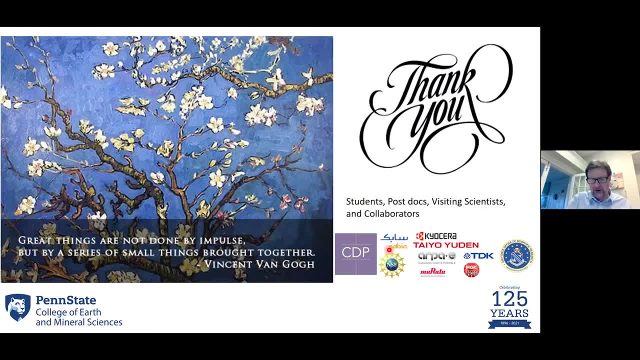 been sponsored by the center for the electrics and peers electrics companies, national science foundation, the air force, and in some of the technologies that we've developed, we've got over 14 companies looking to license this, so these are massive companies that are helping us to then. 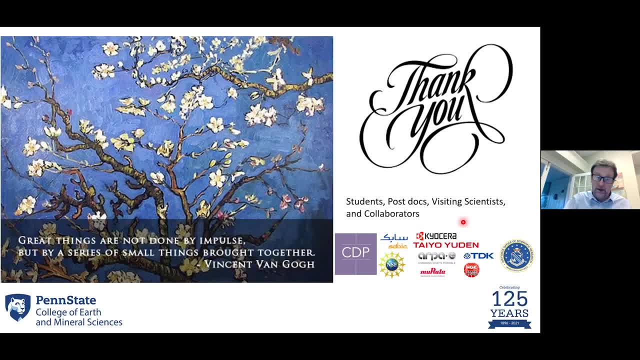 transition this to then benefit society. and remember that most materials breakthroughs take an enormous length of time to go from bench top to society. often, most of the most of the transitions or translations of this materials technology can take up to 15 years. but with very early partnership here, we hope that we can accelerate that process because at the end 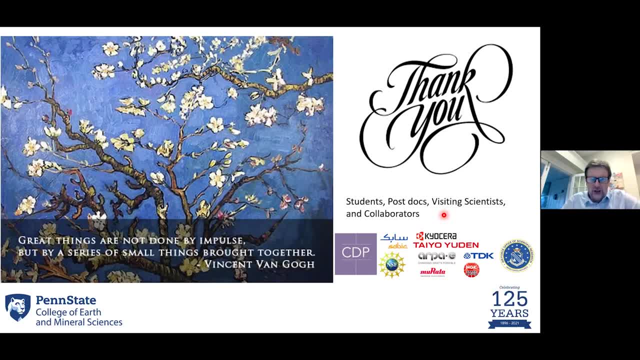 of the day. developing new sustainable manufacturing processes has to be a priority for materials manufacturing and opportunities to then help the um, the energy budgets that we are generating for our society. so i'll leave you with the thoughts of vincent van gogh: great things are done not by impulse. 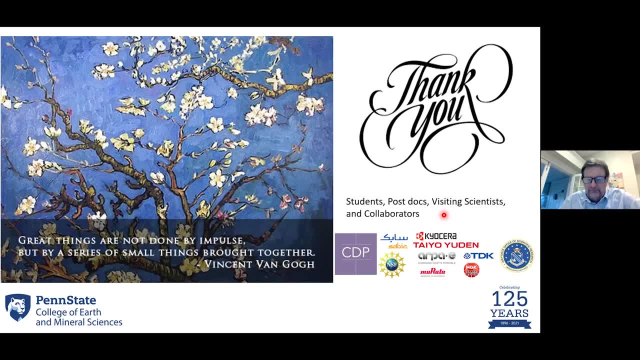 but by a series of small things brought together. so thank you very much for your time. thank you, clive um. so we're going to get started with the question and answer portion. um. one of the first questions that came in is about: how do you think about? 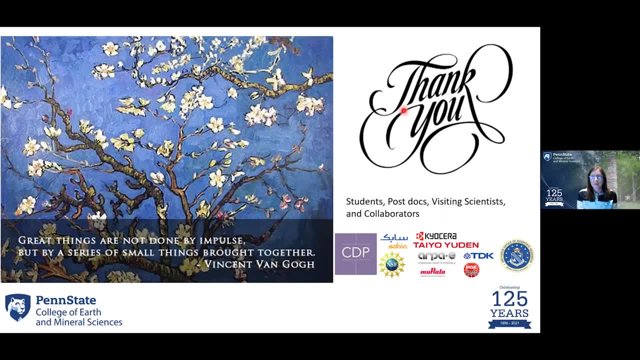 how? this is fascinating, how there's a low temperature process that can build a material or a product in ten minutes. um wondering: are we past the r? d phase to commercialization for any type of product? so um, not yet. we've um. both dr mckinstry, susan mckinstry and myself had a project. with a company that i probably can't give the name of, but it was a buyer voucher that we were just asking. don't talk about the $20,000 cash offer on something i'm bringing you to faces today. what did you wanna do to ensure the concept of artists, what to do to get aС they're out for something i'm so concerned about $20,000 int? 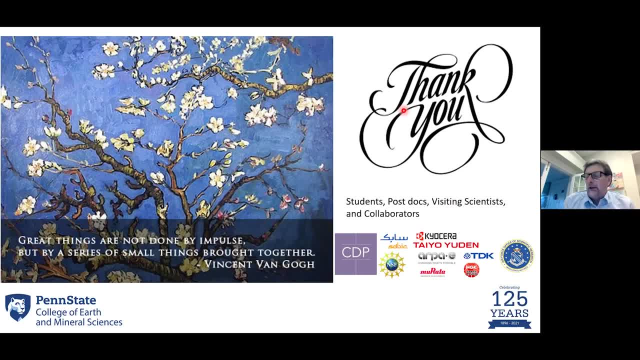 the name of, but it was a biomedical company And we thought that we had a demonstration that they were going to buy into. They sponsored the work. They even patented the work in partnership with us, But that didn't happen. There are other companies that are buying into the license And 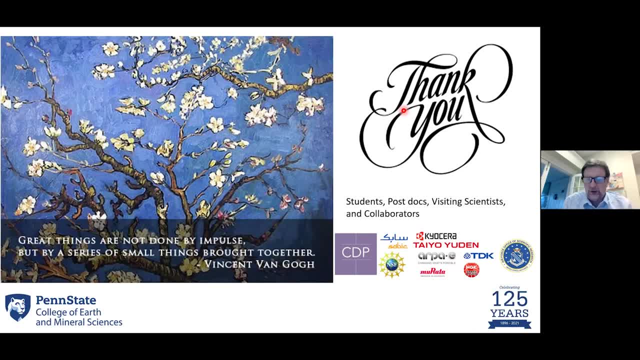 some of them have been visiting scientists from some of the Japanese companies that have worked with me to help with some of the development of this. They've gone back to their respective companies and are working towards that end, And so it is beyond the R&D stage. I would say that 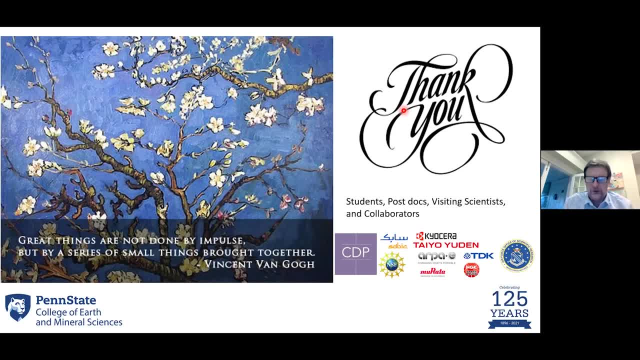 it's in some places at the pilot level, which is really exciting. I guess a follow-up to that would be: which industry or specific type of product do you think we expect to see this come out first using the cold centering? Yeah, I think because I'd worked so closely with the electronic ceramic type companies. 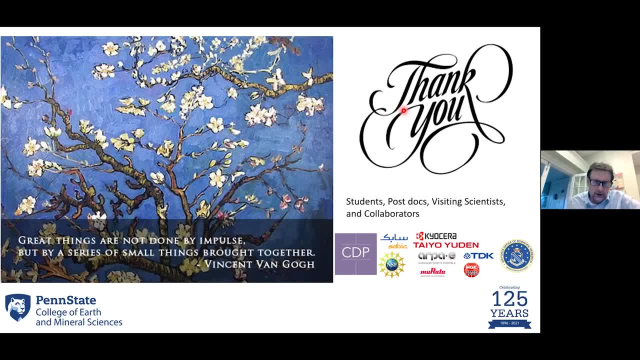 the ones that were aware of it earlier than others because of the work being done in the Center for Dielectrics and Piezoelectrics. So they basically had a four to five year, three to four year jump on this. And then there are also some, you know, they're often highly valued products And so the profit. 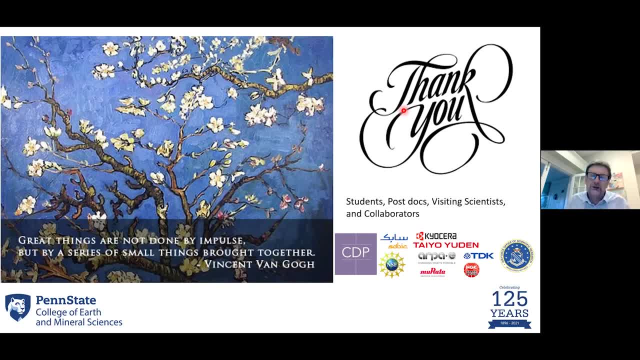 margins are a little bit different from, say, bricks and other things like this. We also have very recently published some work with some of our colleagues at Dubois University, at Dubois Penn State campus, And there we've been able to translate this process to metals. 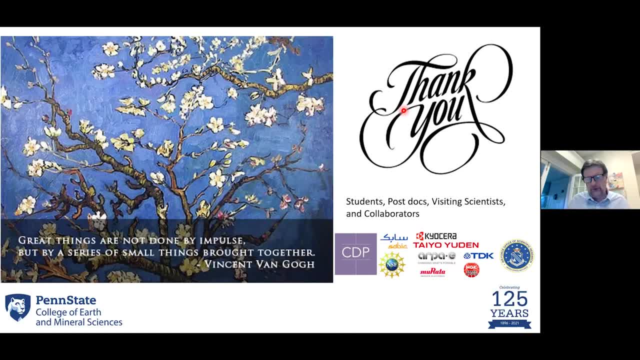 And already some very, very large parts have been made in a powder metallurgy company And almost within the production line that was already in place for traditional powder metallurgy. So we're quite excited about that as we go forward as well. So it's very much happening on multiple fronts. 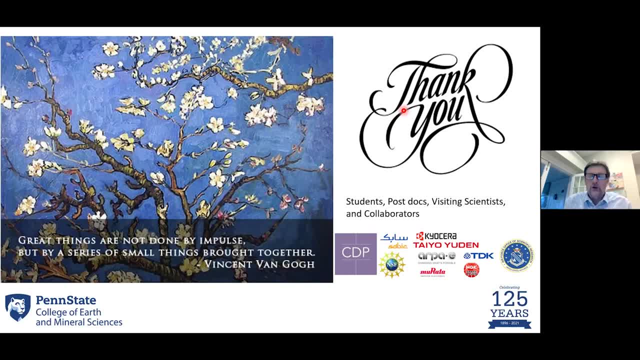 And we still continue to do R&D research. We still don't fully understand all the mechanisms, but the true value of this will come in in the early applications to come forward. So I think it's gonna be electronic ceramics, but it may be metals based. 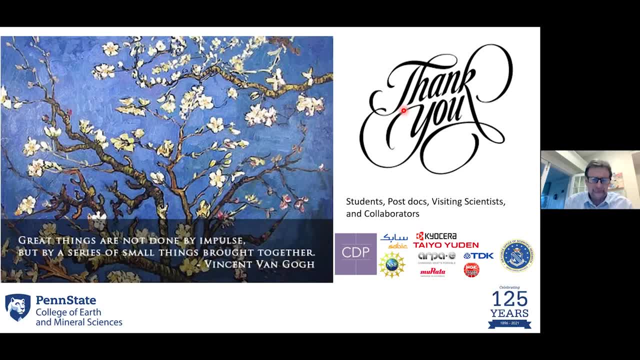 upon how fast that particular area has moved. Debby Lewis: Alright, A question that kind of came in is of the problems with structural ceramics. is the cost associated with the need for high temperature sintering. what is the prospect of this methodology being applied to carbide nitride and boride? 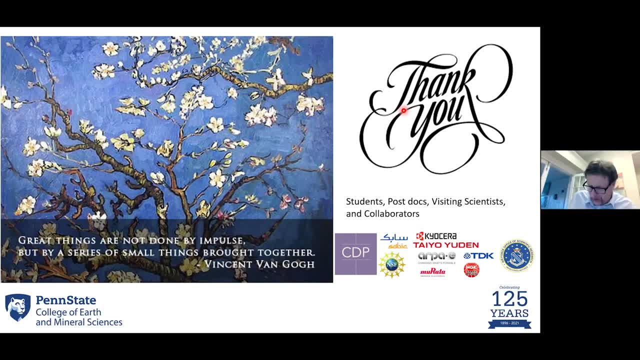 ceramics. yeah, so that's a brilliant question. that's uh, we've asked ourselves many times before and, um, what i will say in terms of the structural materials, ignoring the the chemistries that were just said, is that we've successfully had some very good results with zirconia. now, that's not. 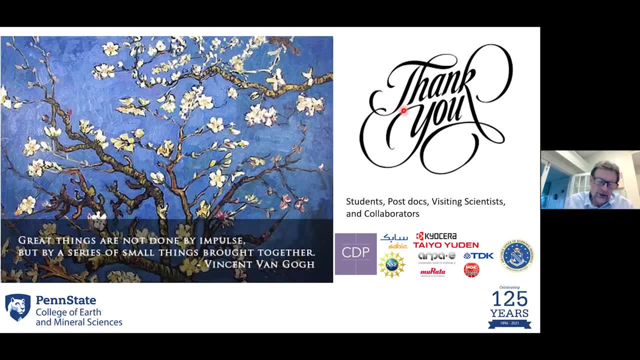 a nitride or a carbide and um, and i think the process is absolutely ubiquitous, but really what it takes is a very, very good chemist to understand these interfacial reactions and i think we need to have chemists that really understand carbide and nitride, um, surfaces and solvents and um. 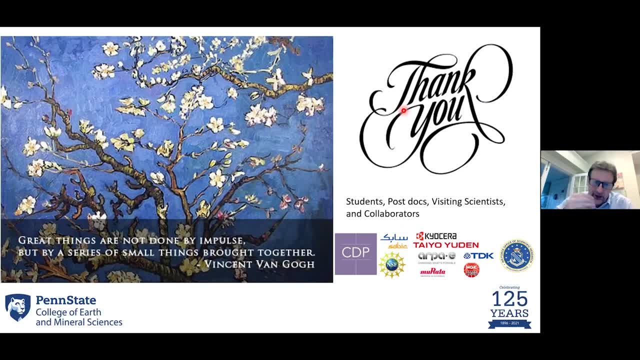 and maybe metal organics solvents that that could then drive the dissolutions process for aluminum or silica in those types of materials. at this point i do not know how to do it and it's not obvious how to do. how to do that, um, but you're right, structural materials are very interesting. 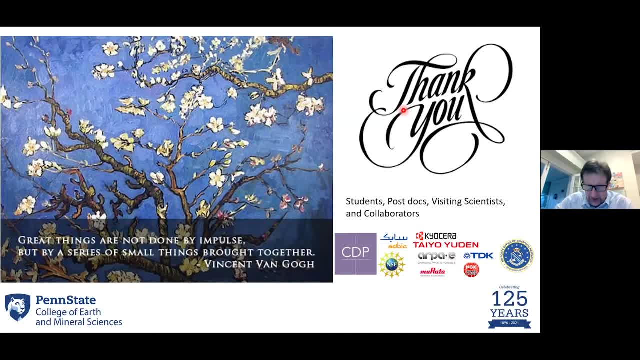 i know that we could do it in zirconia, the, the covalently bonded aluminum nitrides and carbon bides, etc. that's a tough rate to correct. it needs a clever chemist. um. can the us provide all the materials necessary for the low temp process? 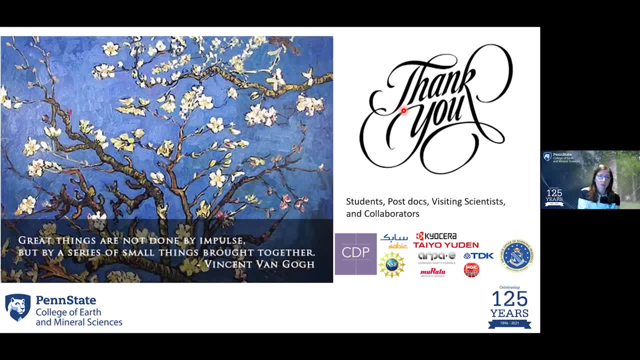 or does this require us to continue to import raw material? yeah, that's, that's also a very good question, right? um, i mean, um, interestingly enough, there is some, uh, we've had some. some of my students are very creative and i've had one of my students uh reach out to um, some of the mining waste that is there. 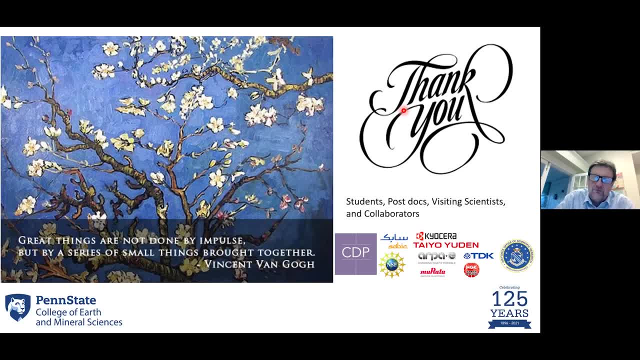 in york county and um he's made some very, very primitive but good looking brick structures. i mean not large bricks are making one at a time, but but tile like structures out of some of that waste that is coming out of the mining waste. and i think that's a very good question and i think 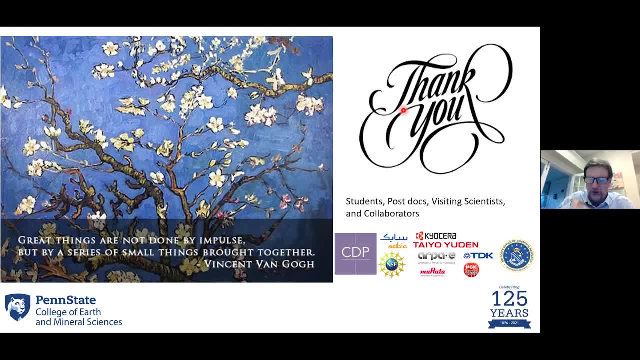 this is one of the things that i've been interested in is that um um the original m 1962, 2019 yeni early Birthedge to a factory here in the US. So until we get enough and drive the cyclic economy, I think we're always going to be somewhat dependent upon those. 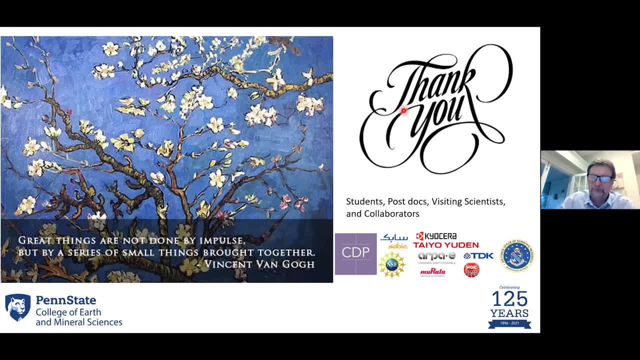 even if everything which we've talked about here comes true. So I guess, moving, continuing with the cyclic economy, does low-temp sintering enhance the ability to recycle lithium batteries, For example, enhancing the viability of this battery technology? Yeah, that's obviously an area where we think you do have the value added. 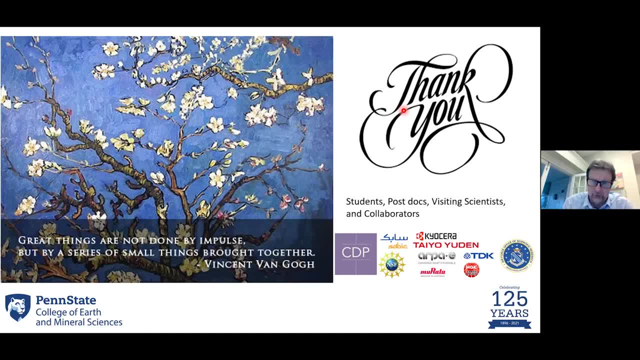 where you can actually recover a lot of those materials, the cobalt and basically the lithium cobalt or the manganese, the nickel, manganese, cobalt type formulations, and then basically recover them And then you can recycle them if the lifecycle analysis allowed you to bring enough. 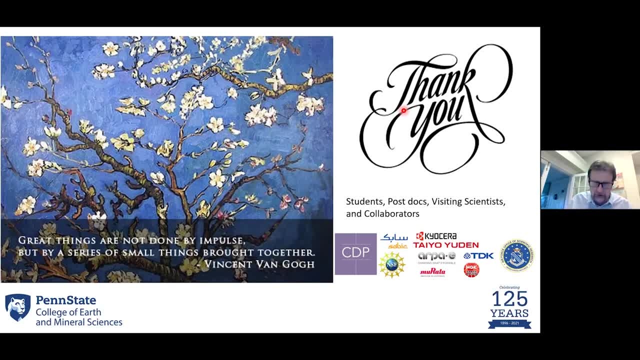 together to then actually give it as a net gain. But in principle, yes, The battery area is a very good one. We've got a number of people working in that space. What is the typical composition of the liquid phase? Does the production of the liquid phase negate any significant 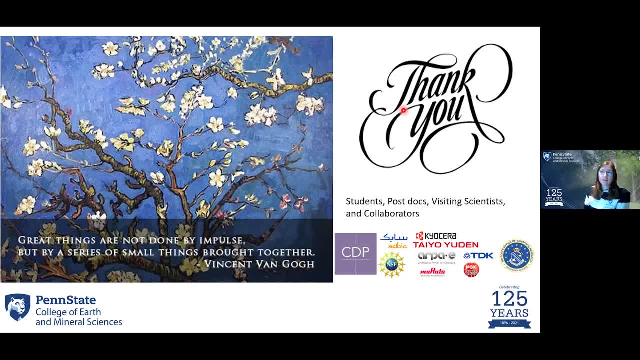 portion of the energy savings. Yeah, the liquid phase is critical. It doesn't have to be much, by the way, It can be just a few percent by volume, but it has to allow for the control of congruent or near-congruent dissolution. 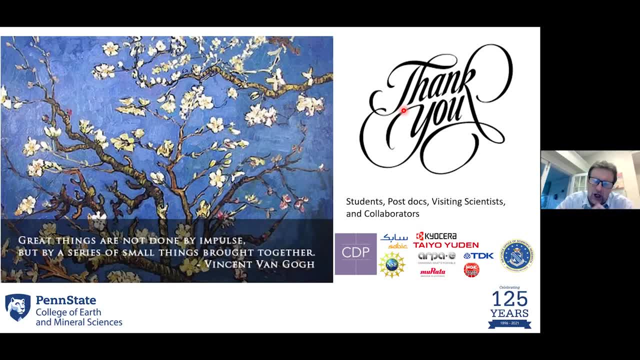 So you're balancing the chemistry at that surface And so designing. that is a lot of the tricks that has to be thought through, particularly for more complicated chemistries where it's very easy to have differential dissolution rates In some of the batteries, for example. 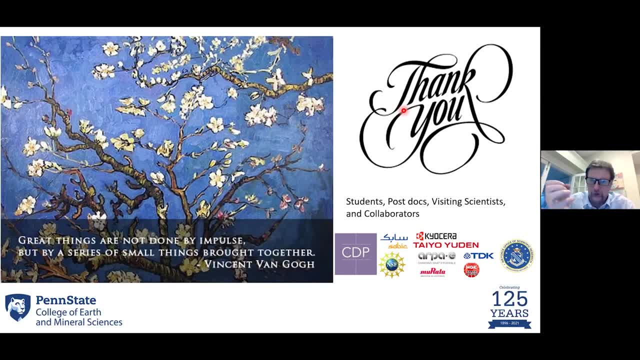 we've got just polar solvents and more simpler materials, good on water, acid-base chemistries to then drive the dissolution kinetics is also what we use. So we use general chemistry, principles of dissolution, but the ability to then control all the speciation. 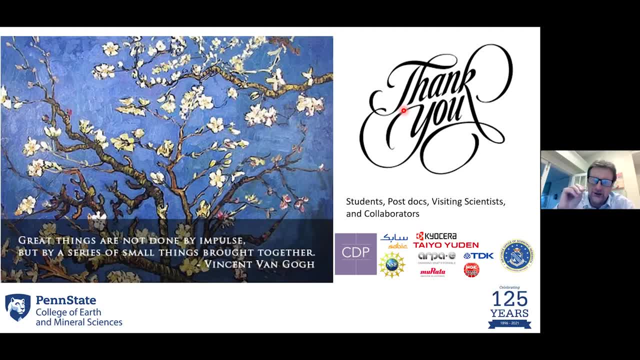 that you need to get into the solution and precipitate out is the work that you have to do to really make sure that you're developing the stoichiometries that you need. And obviously some of the materials in batteries have three to four chemical components. 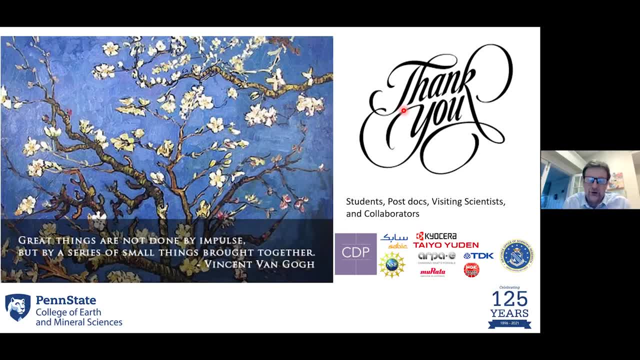 so they become a little more trickier to control than, say, I don't know zinc. I don't know if it's zinc oxide or magnesium oxide or zirconium. So are you working on any other processes besides low temperature? Is the federal government funding the research? 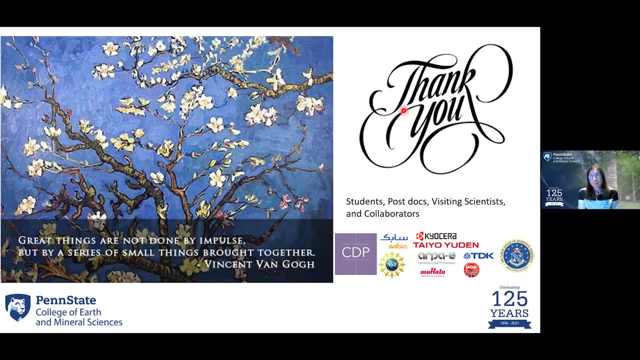 or do the funds come from the private-public sector? Both I have funding from both the federal sector and also from companies, And I'm working on other processes. I mean, I've always dabbled with processing. I was trained as a physicist. 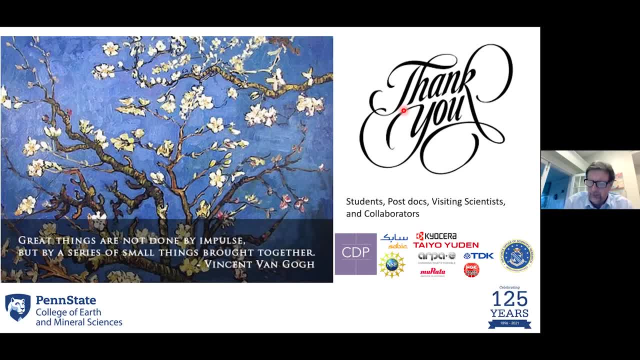 so I didn't really regard myself as a processing-type person, But over the years we've developed some things. In fact, probably my biggest breakthrough, which I didn't patent, was a fast-fire process for capacitors, of which there's probably $3 trillion of them made a year. 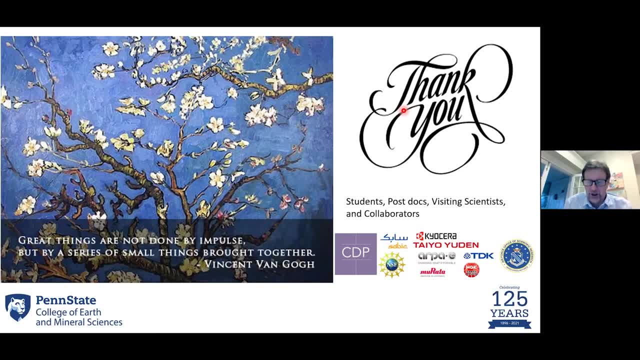 And I was more interested in the thermodynamics and the kinetics of that than I was the patent, which was probably a mistake for Penn State and myself, Never mind Continuing, I guess, with other companies or industries involved in the process. how many other universities are working on the same technology? 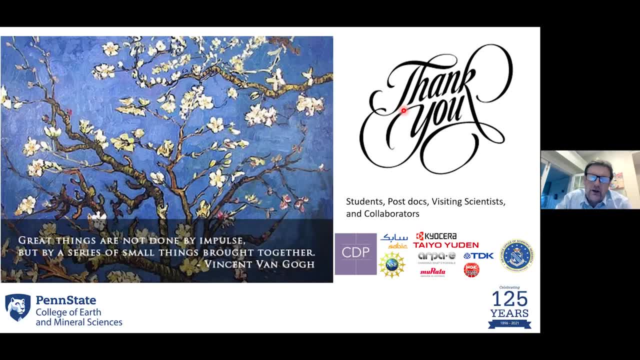 Yeah, so it's expanding. Certainly we've had people from Europe. We've had people from Japan- Japan- That we've trained in the labs here. They come over for three or four months to then just see what we're doing. 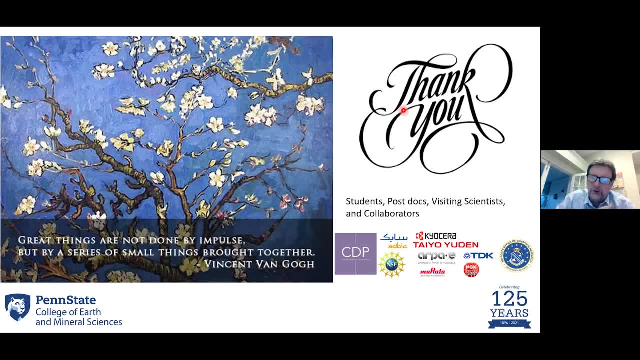 And programs are building up around the world. We need that because you know, we have one idea. I mean even colleagues at Penn State here: Dr McKinstry, JP Maria Enrique Gomez- I already mentioned, and others have all looked and duplicated what we've done. 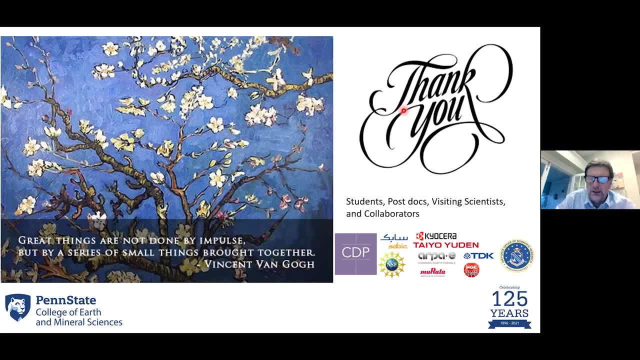 and expanded new ideas to how to proceed forward, And so, As you know, it's going to take a community to then really develop all the skill sets that we need to be able to make a big difference with this type of technology, And you need people who are much better chemists. 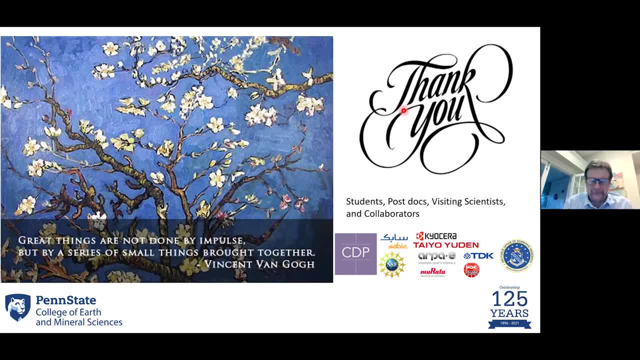 as I pointed out, than myself to drive this, And I guess a follow-up to that would be- and then you have maybe mentioned it is: how long have you specifically been working on developing this process And or how long has you know? 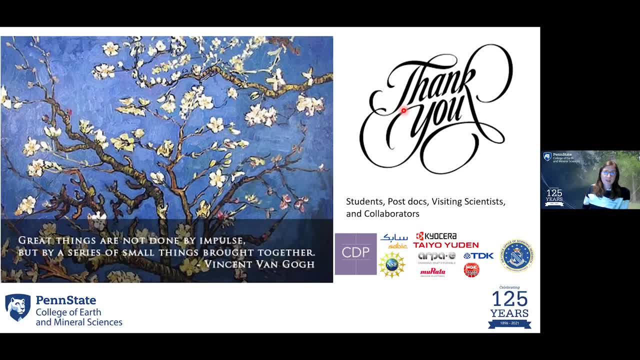 ceramics been trying to get to this process. I think there's always been an element of trying to work with low temperatures. The Japanese in the 1970s looked at hydrothermal searing, which was a closed system. We have an open system which offers you a lot more. 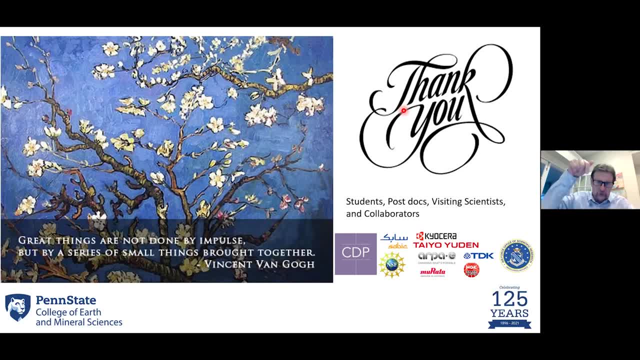 and in the hydrothermal system. it's a closed vessel and you know the liquid gets in the pores and it then minimizes the shrinkage densification processes. So in the 1970s we really started in around 2014,- 2015,. 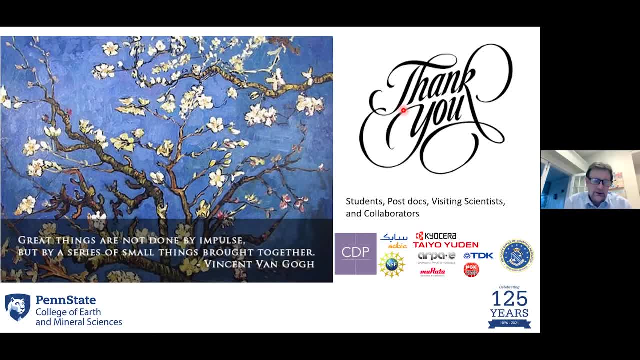 and I was inspired by a paper out of Finland where where, basically, it was to me it was very clear because of all the reading that was going on that I'd been doing around reading around geology and so forth. That was absolutely obvious to me what was happening. 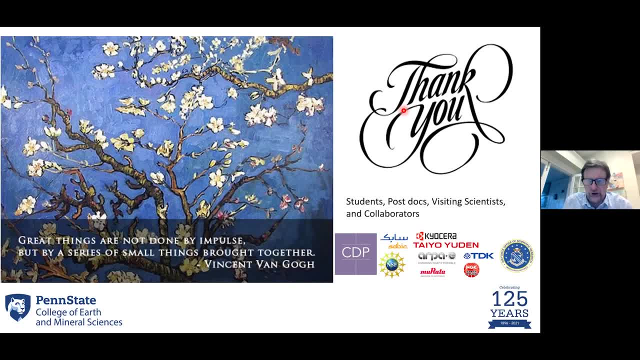 even though they didn't fully understand the mechanisms and how to proceed outside of that one system that they made these observations on, And so we then very quickly got moving, and I think within three months we'd almost done 60 to 80 materials. 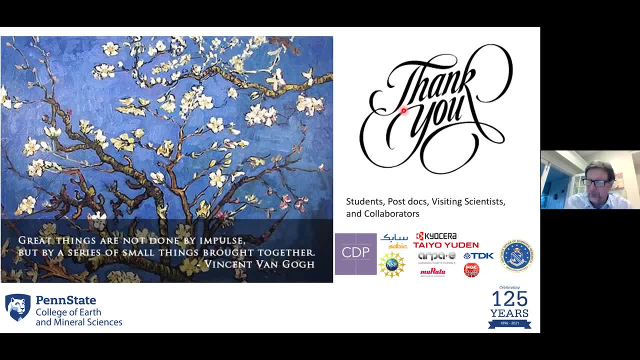 We worked in secret for about two years. I made the first public announcement in France at a meeting in Limoges, And I remember I gave the very first talk at the conference, a plenary, and I think people would expect me to give a very different talk on electronic materials. 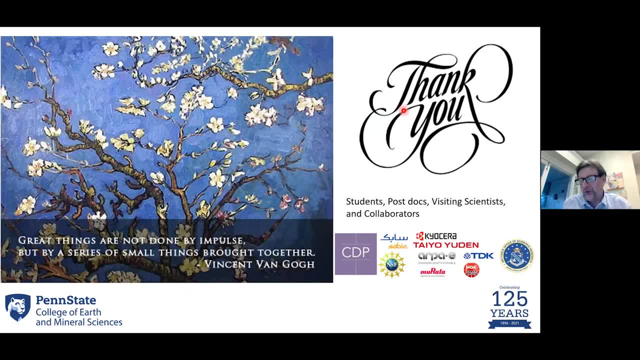 And I think people thought that. in fact, some people joked with me afterwards and said many people in the room did not believe what they saw. In fact, they thought that I was fooling with their minds and just almost giving them fake news. 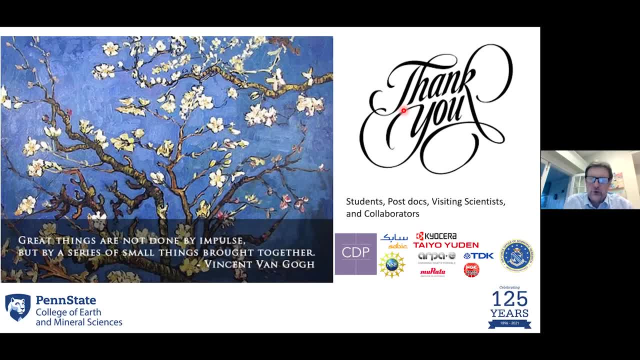 And and but you know, people have duplicated the work, improved upon the work and now a substantial number of groups around the world are working on it. A comment that came in is it would say: A comment that came in is it would say: 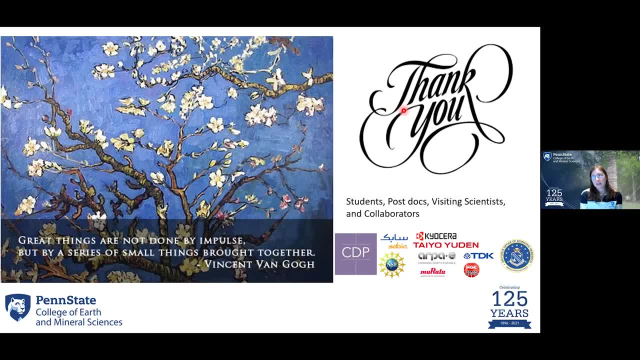 A comment that came in is: it would say: It would seem like the medical industry would be interested in new products that are repeatable, dependable and fit within a tight tolerance and also won't light up an airport metal detector. Yes, 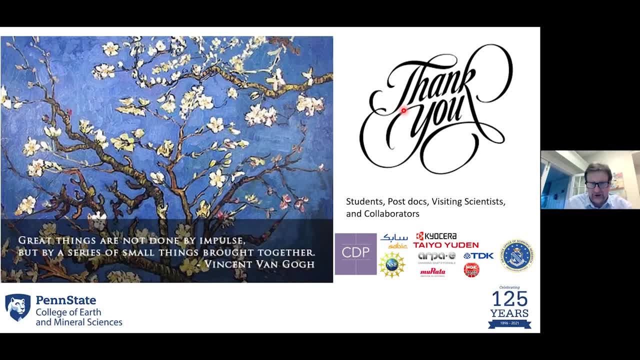 Yeah, so, as I said, one of the applications we were looking for was a medical application, although that particular application wasn't implantable. In fact, a friend of mine at Sheffield who's followed our work very closely and I've guided them- 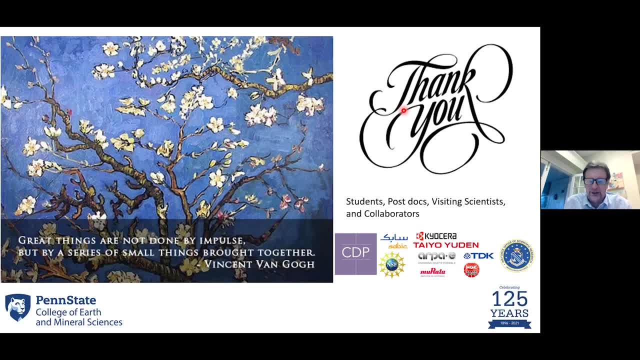 he's doing a lot of work on bioceramics- and he's the one that I talked about in terms of putting living cells into the process, And so that's work that he's really pushing much harder, but he's done a lot of work in bioceramics. 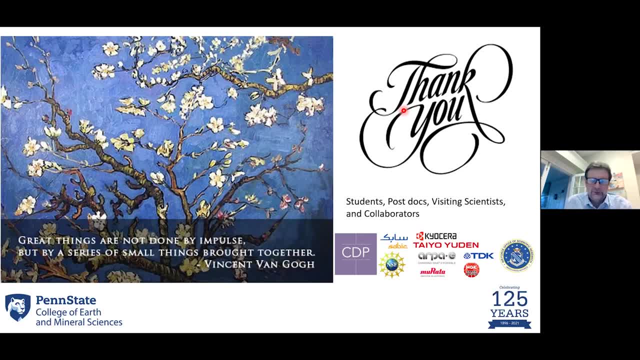 So a question is- and they mentioned- you may have mentioned this before- but what is the fuel source for creating the heat- natural gas or electricity or something else? It's just, in fact, we're doing things with a local electric heater. 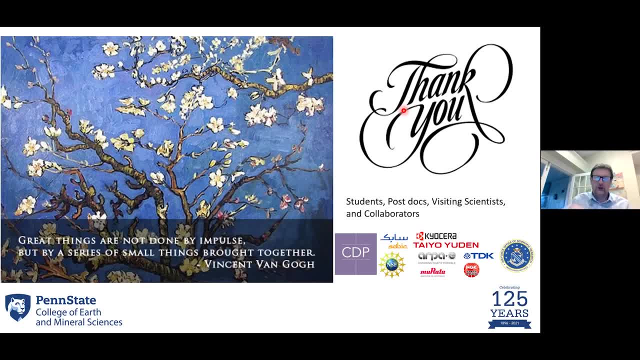 And so it's just heating the fixture which you're pressing into. We design it so it has most uniform heat and we can drive it at different rates. Some of the heating rates can be as high as 25 degrees a minute, And we see advantages of even being able to control the non-isothermal heating rates. 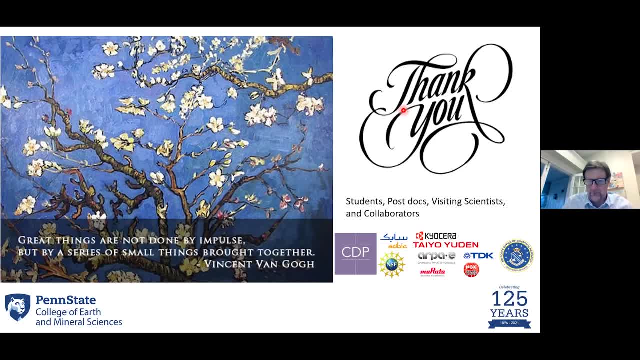 in terms of designing the microstructure and the final products in a number of different cases. So, are you going to do you have, or do you plan to have, several patents on this low-temperature process? Yeah, we have a very strong, very first patent. that's now. I think it's been. 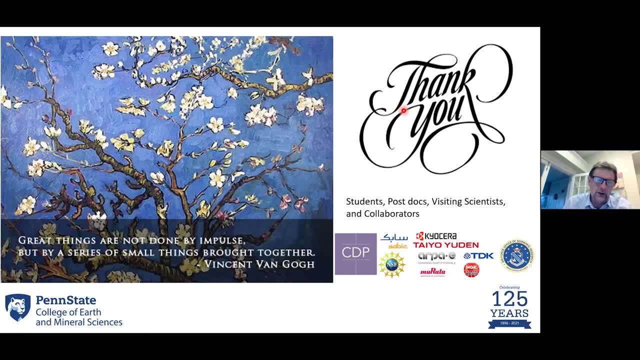 it's got two acceptances for international patents as well, And there's another six being processed, So will this process primarily replace current manufacturing processes, or will this be equally applied to new material design? Yeah, that's a good question, I think, because some of the bigger furnaces can load many, many more pieces. 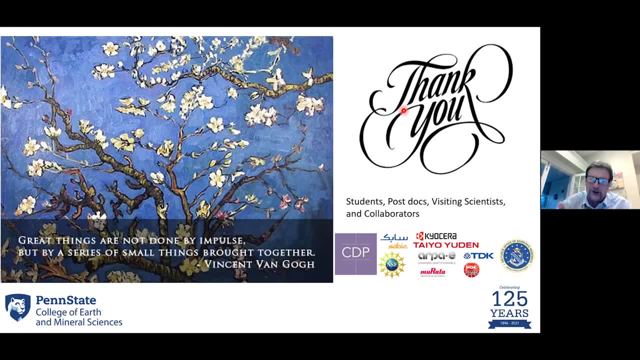 this is why it's critical for us to find ways of doing continuous processing with this, And that's another big challenge, That's another big jump that we've got to make Until we have a continuous process with very, very high-quality parts. 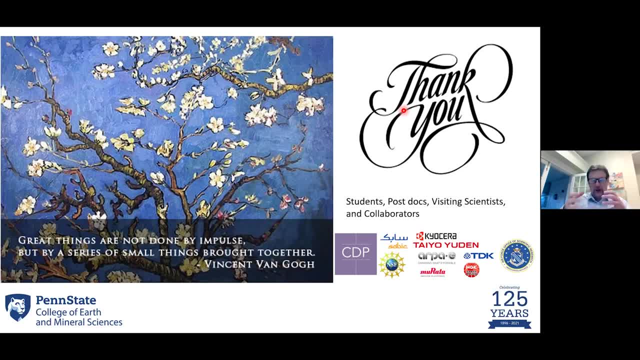 I think you're going to be left with batch-type processing. So actually I said we're looking at batteries. I'm very interested in sodium batteries for you know, the same way as you may make fuel cells, and just basically. 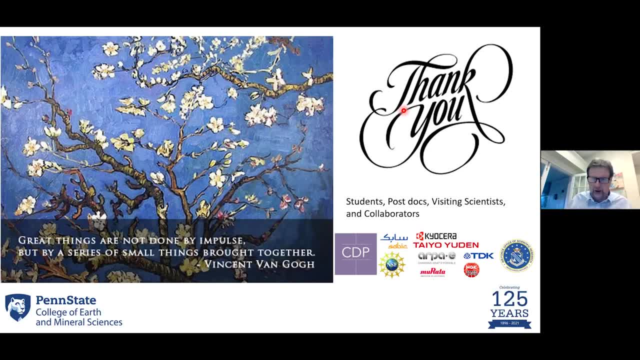 Build things on a batch-like basis and then fire them and then try and push them along in that way. So there are hot pressing factories, There's factories that do hot pressing and you have a whole floor of batch processes. Some of those types of applications we see is one of the ways forward. 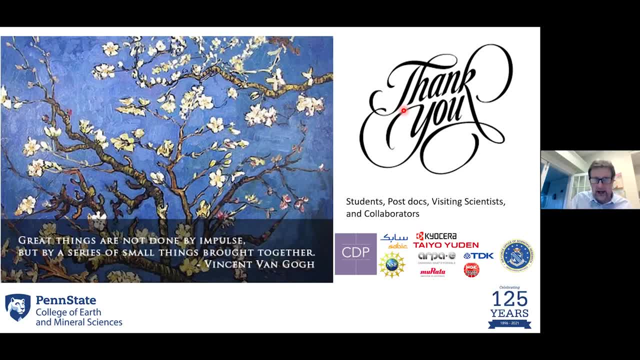 That's why I was very, very pleased to see this. you know, dropping the powder metallurgy cold sintering approach into a present manufacturing line And then developing much better properties, with just adding these wonderful transient phases Moving into the university impact. are you at a stage where this can be incorporated into undergraduate curriculum? 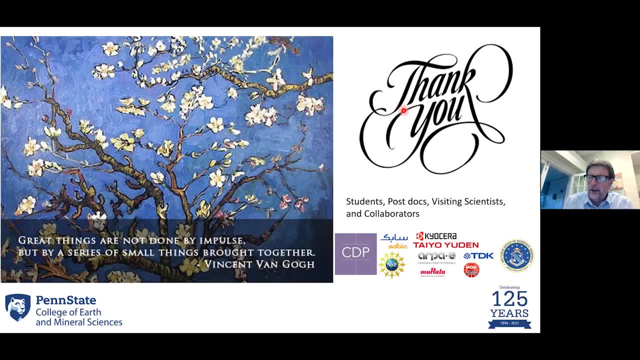 Yeah, it certainly could be. I know an expert in STATA that's a faculty member. I know an expert in STATA that's a faculty member. A faculty member at Georgia Tech basically built it already into a design course and got NSF money to do that. 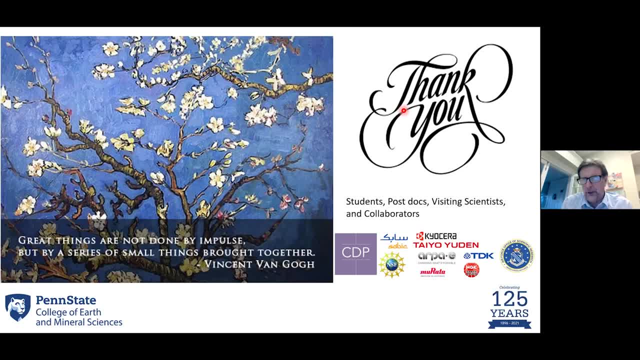 A friend of mine who was writing a book on ceramic materials dedicated a part of a chapter at the end of the book for the future of ceramics, where he dedicated a large part of that chapter to cold sintering. So and that's an undergraduate textbook. 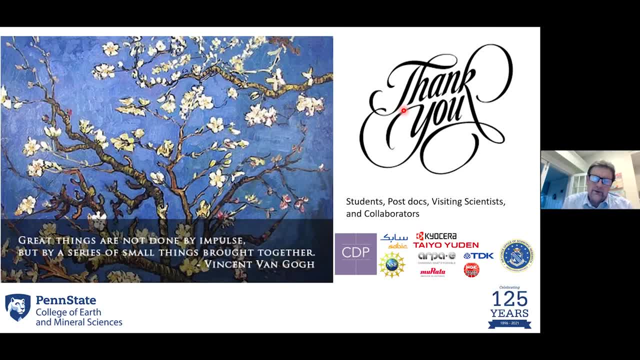 And so I do think that the educational part of this is still developing, because we don't fully understand it, But I think it's a very in fact, one of the beauties of this is actually, you know, in principle, you could do it in your garage, right? 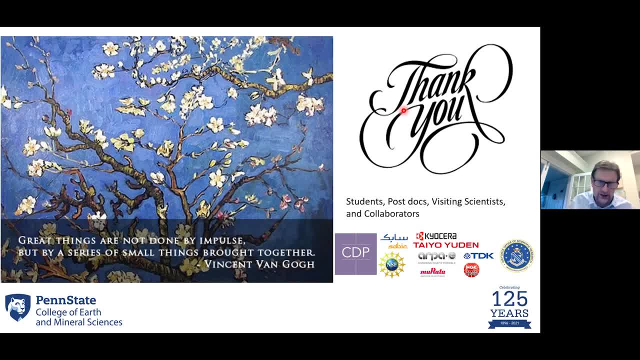 You don't need to have a big furnace to do this. You can make a ceramic within 10,, 15 minutes And all you really need is a press and a small heater And you put the powder together, do your powder processing, get it to work and you've got a dense ceramic. 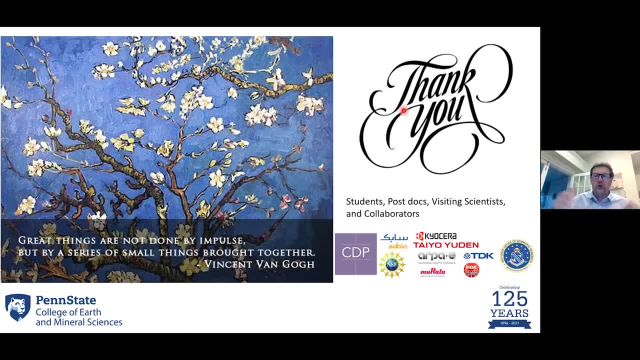 Any of us that have done pottery know that. you know there's a long process of where you lose the pot it goes, and then you get it a couple of days later. So to instantly see that that return on your processing I think is also very exciting for people undergoing the education mission and learning more and more about materials. 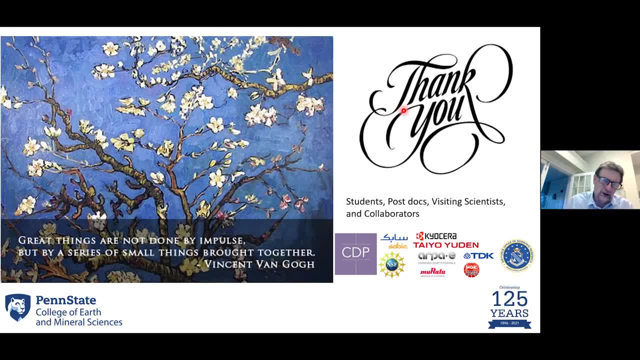 It can also be a process that can be taught and introduced into under-resourced communities as well. In fact, I've given talks at the African MRS meeting, for example, on this subject And it's possible potential for some of the brick making skills and processes that they have in places like Tanzania. 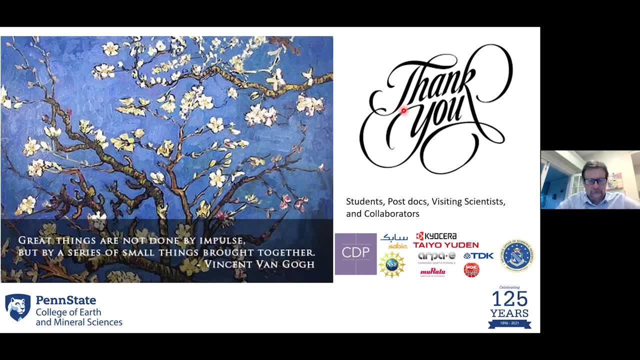 Thank you. So for cold-centered ceramics, would the electronic or other properties be similar? Would this process produce materials with even better properties than conventional process? Yeah, so I think mechanical properties are down a little bit, But electrical properties, especially when you're putting polymers in the grain boundaries. 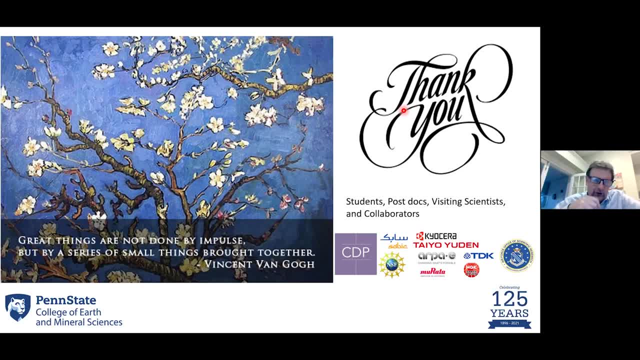 I've worked on dielectric materials for over nearly 25 years plus, And very recently We've been able to design dielectrics in ways that I never thought you could do it, And it's much better than what you can do with all the conventional methods. 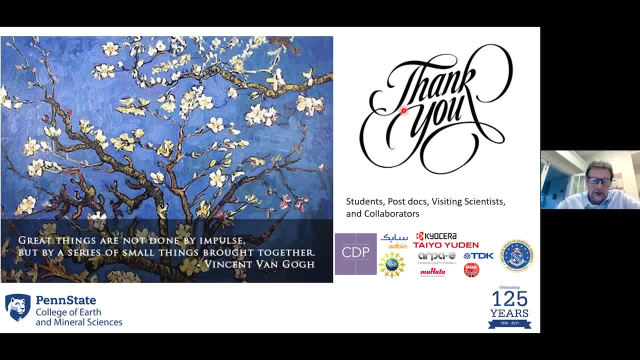 They would be more reliable, They'd be able to withstand higher, They would have higher breakdown strength And they also have very, very good properties at high fields And they're able to withstand higher breakdown strength. So they're able to withstand higher breakdown strength. 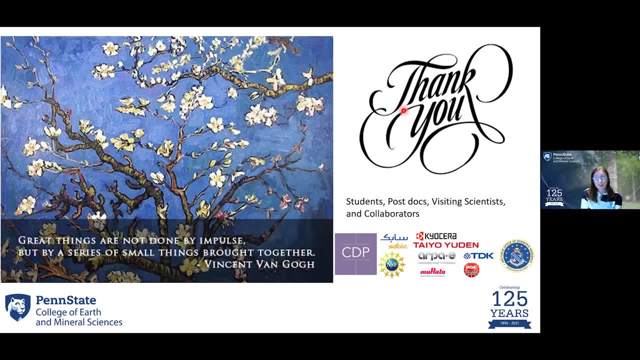 So they're able to withstand higher breakdown strength. A comment comes in saying thank you for the great information. You've created a new methodology to create materials that can be used in many, many industries. Another testament to the expertise that's held at Penn State, especially in the College of Earth and Rural Sciences. 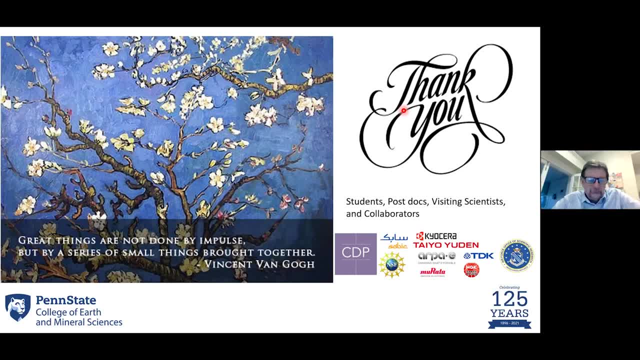 Thank you. Thank you, So our questions and comments seem to have slowed coming in. I'd like to just put a call out for any other last minute questions that people might have Or any comments you'd like to Pass along. You know this has been a really informative talk. 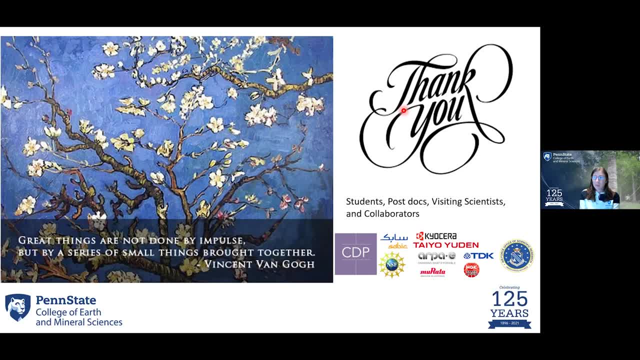 And I think it really touches upon the broad science that EMS participates in. No, I think it offers for the first time a common processing platform for all forms of materials Where a polymer person can work very easily with a metals and ceramics person, And in that was always very.